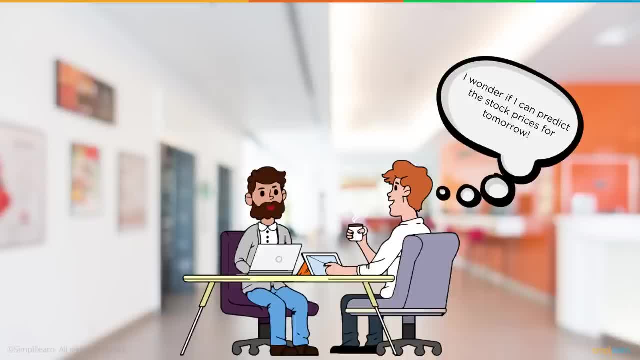 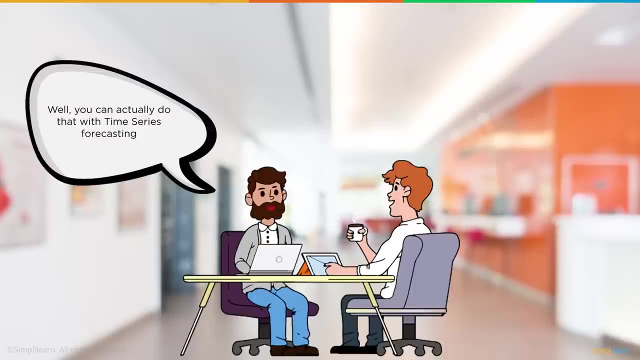 delay, let's get started. and so why exactly do we need to do time series analysis? typically, we would like to predict something in the future, and it could be stock prices, it could be the sales or anything that needs to be predicted into the future. that is when we are going to be doing time series analysis and we are going to be doing time series analysis. 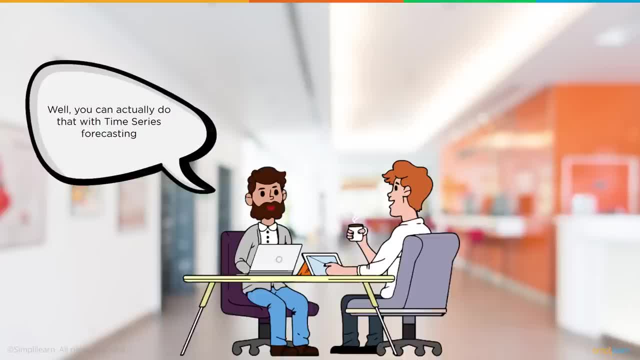 and we use time series analysis. so it is as the name suggests, it is forecasting, and typically when we say predict, it need not be to the future. in machine learning, in data analysis, when we talk about predicting we are not necessarily talking about the future. but in time series analysis we 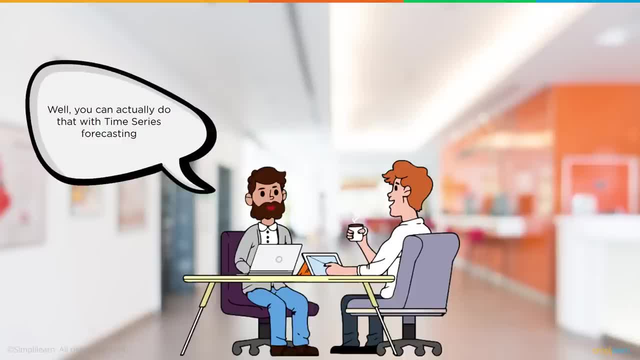 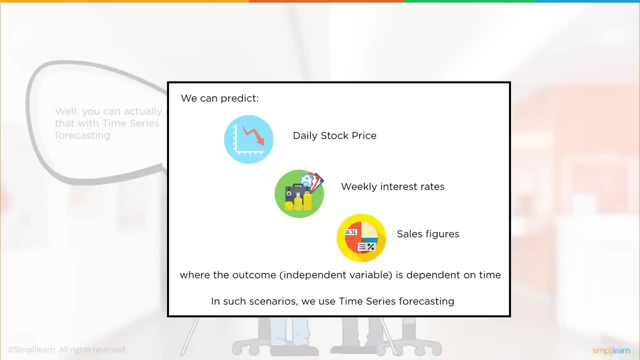 typically predict the future. so we have some past data and we want to predict the future. that is when we perform time series analysis. so what are some of the examples? it could be daily stock price, the shares as we talk about, or it could be the interest rates weekly. 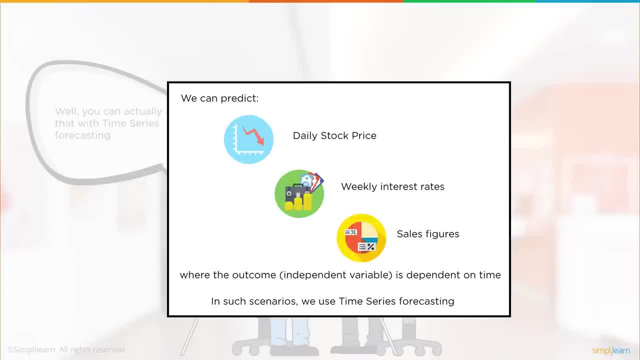 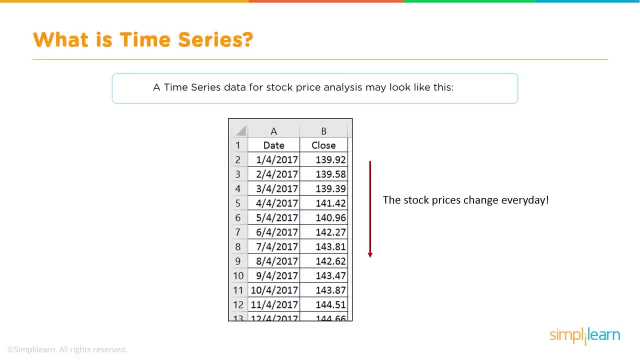 interest rates or sales figures of a company. so these are some of the examples where we use time series data. we have historical data which is dependent on time and then, based on that, we create a model to predict the future. so what exactly is time series? so time series data has time as one of. 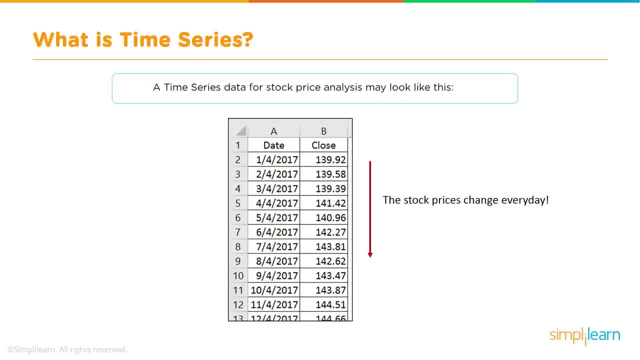 the components, as the name suggests. so in this example let's say this is the stock price data and one of the components. so there are two columns here. column B is price and column A is basically the time information. in this case the time is a day, so that primarily the closing price of a particular stock has been recorded on a daily. 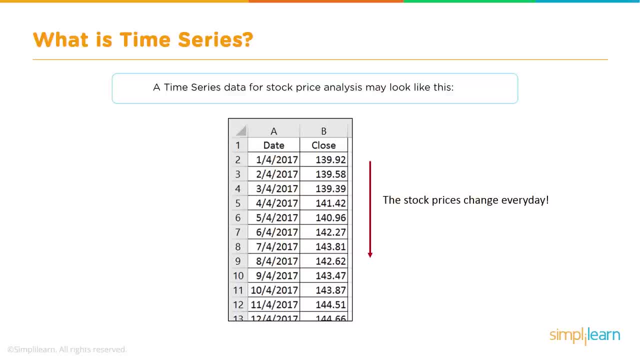 basis. so this is a time series data and the time interval is obviously a day time series or time intervals can be daily, weekly, hourly or even sometimes there is something like a sensor data. it could be every few milliseconds or microseconds as well, so the size of the time intervals can vary, but they are fixed. 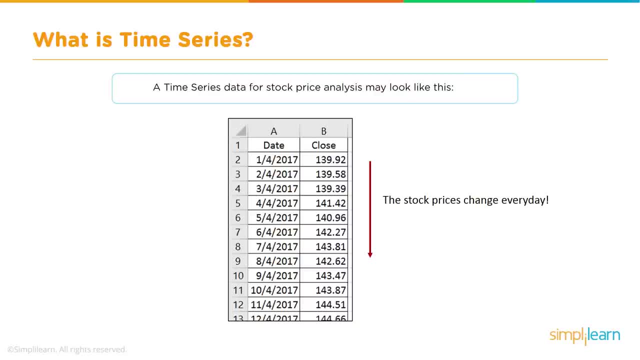 so if I'm saying that the it is daily data, then the interval is fixed as daily. if I'm saying: if this data is an hourly data, then it is. the data is captured every hour and so on. so the time intervals are fixed. the interval itself you can decide. 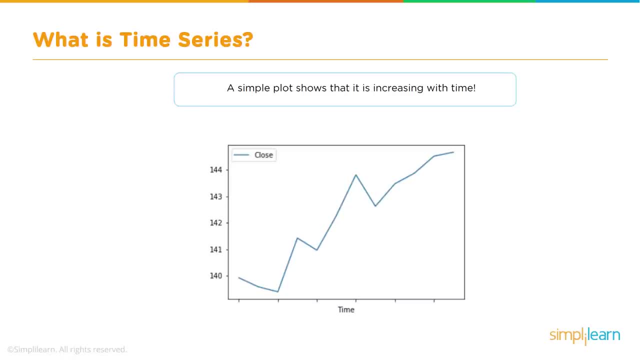 based on what kind of data we are capturing. so this is a graphical representation, the previous one here we saw the table representation and this is how the plot the data. so on the y-axis is, let's say, the price or the stock price and x-axis is the time. so against time, if you plot it, this is: 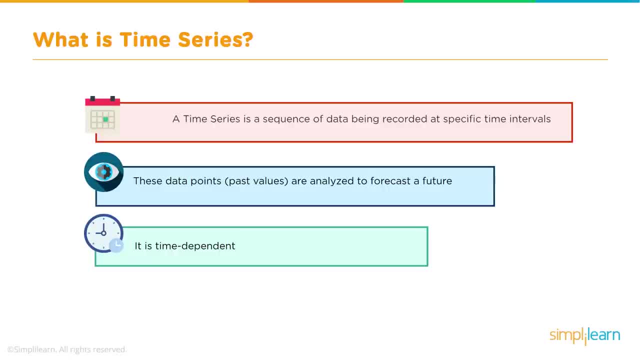 how a time series graph would look. so, as the name suggests, what is time series data? time series data is basically a sequence of data that is recorded over a specific intervals of time and based on the values. so if we want to do an analysis of time series pass data, we try to forecast a future and 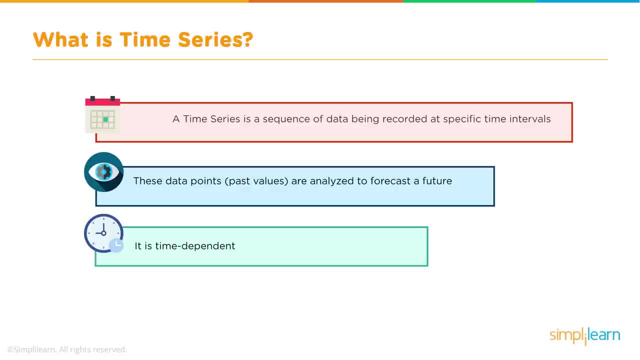 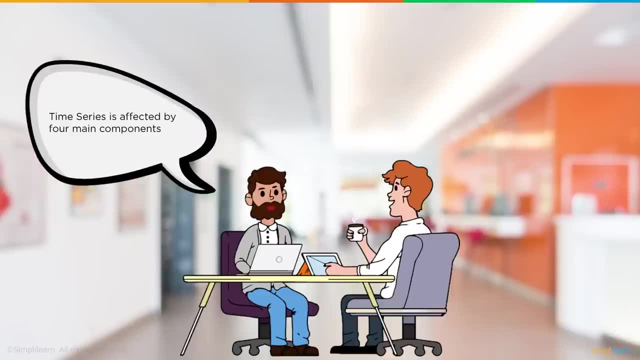 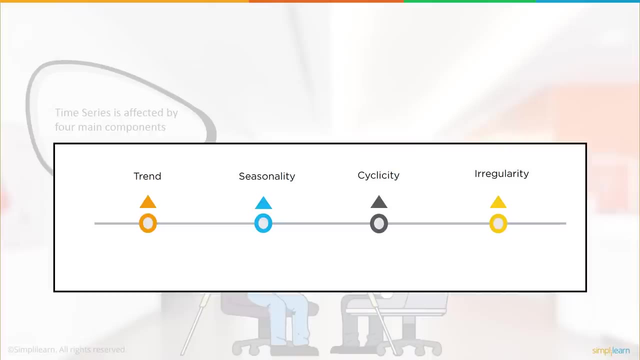 again, as the name suggests, it is time series data, which means that it is time dependent. so time is one of the components of this data. time series data consists of primarily four components: one is the trend, then we have the seasonality, then cyclicity and then, last but not least, irregularity. 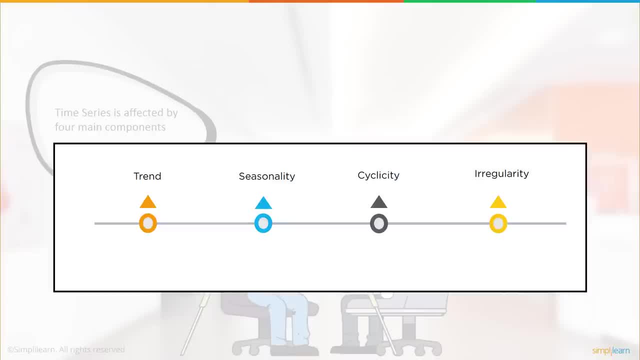 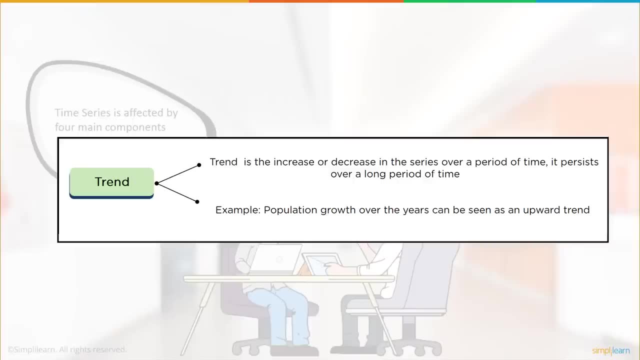 or the random component. sometimes is also referred to as a random component. so if you want to do an analysis of that component, so let's see what each of these components are. so what is trend? trend is overall change or the pattern of the data, which means that the data may be. let me just pull up. 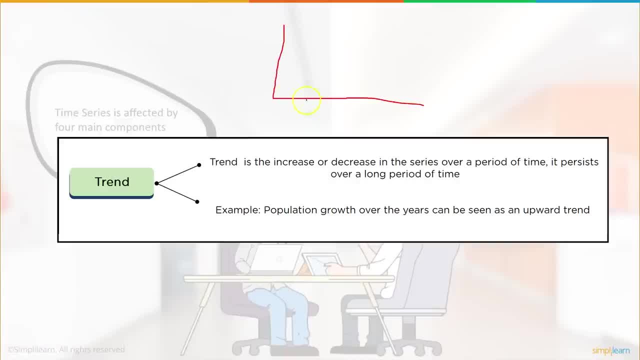 a pen and show you. so, let's say, you have a data set somewhat like this, a time series data set somewhat like this. all right, so what is the overall trend? there is an overall trend which is upward trend, as we call it here. right, so it is not like it is continuously. 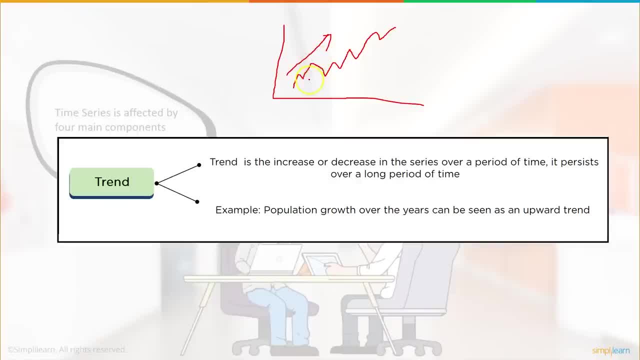 increasing, there are times when it is dipping, then there are times when it is increasing, then it is decreasing, and so on. but overall, over a period of time, from the time we start recording to the time we end, there is a trend right, there is an upward trend in this case, so the trend need. 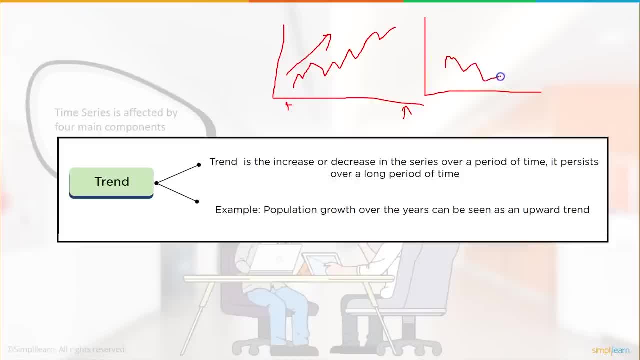 not always be upwards. there could be a downward trend as well. so, for example, here there is a downward trend, right? so this is basically what is, uh, a trend overall, whether the data is increasing or decreasing. all right, then we have the next component, which is seasonality. what is seasonality? seasonality as: 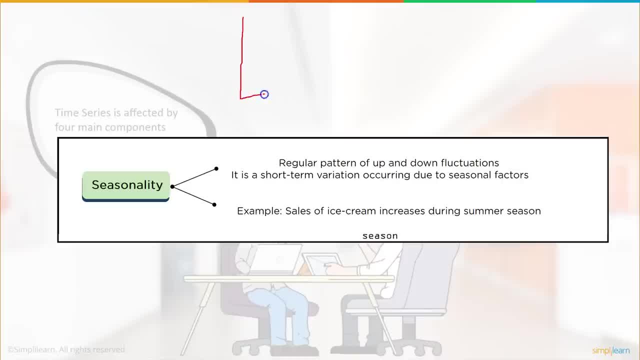 the name suggests once again changes over a period of time and periodic changes. right, so there is a certain pattern. let's take the sales of warm clothes, for example. so if we plot it along the months, so let's say January, February, March, April, May, June, July, and then let's say it goes up to December. okay, so this is our. 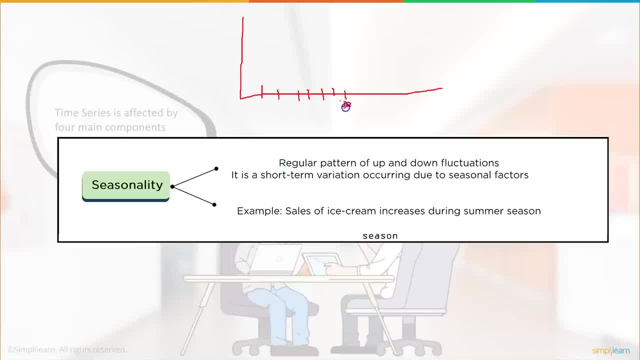 December AD- I will just mark it as D. and then you again have Jan, Feb, March, and then you get another December. okay, and just for simplicity, let's mark these as Decembrists, as the end of the year, and then one more December. okay, so what will happen when? if you're talking about 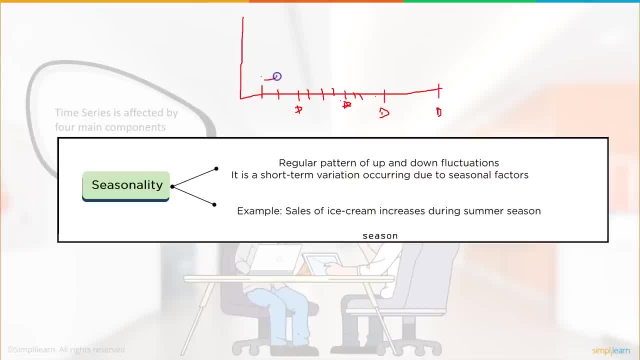 warm clothes. what happens? the sales of warm clothes will increase, probably december when it is cold, and then they will come down, and then again around december again they will increase, and then the sales will come down, and then there will be again an increase, and then they will come down, and then again an increase, and then they will come down. let's say this is: 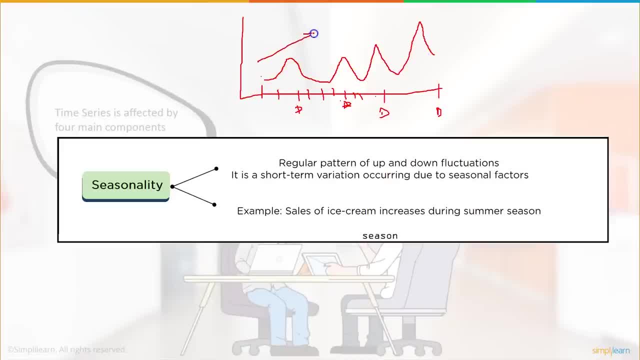 the sales pattern. so you see, here there is a trend as well, there is an upward trend. right, the sales are increasing over. let's say, these are multiple years, this is for year one, this is for year two, this is for year three, and so on. so for multiple years, overall, the trend there is an upward trend. 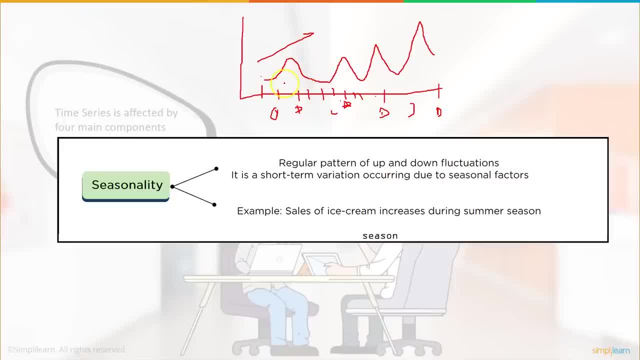 the sales are increasing, but it is not a continuous increase, right? so there is a certain pattern. so what is happening? what is the pattern? every december, the sales are increasing, or they are for that particular year, right. then there is a new year again. when december approaches, the sales are. 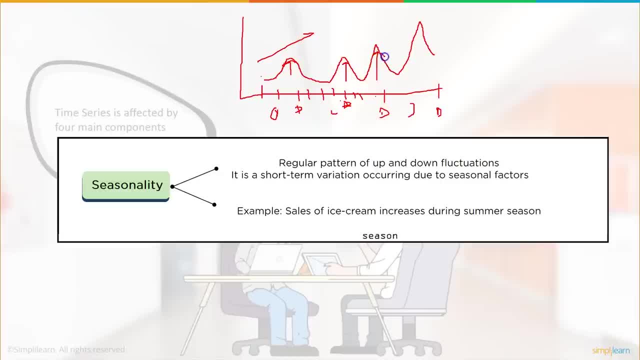 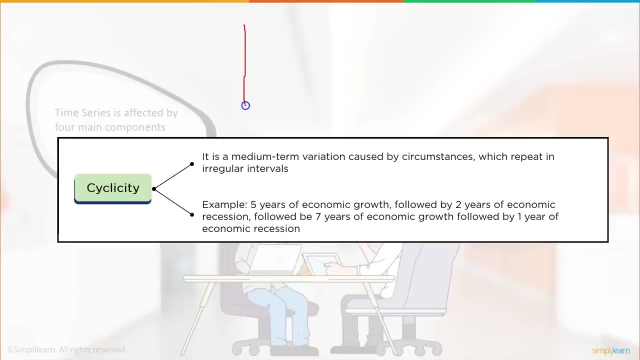 increasing again. when december approaches, the sales are increasing, and so on and so forth. so this is known as seasonality. so there is a certain fluctuation, which is which is periodic in nature. so this is known as seasonality. then cyclicity: what is cyclicity? now, cyclicity is somewhat similar to seasonality, but here the duration between two. 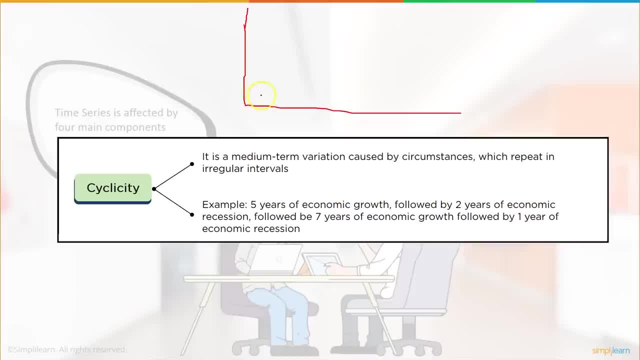 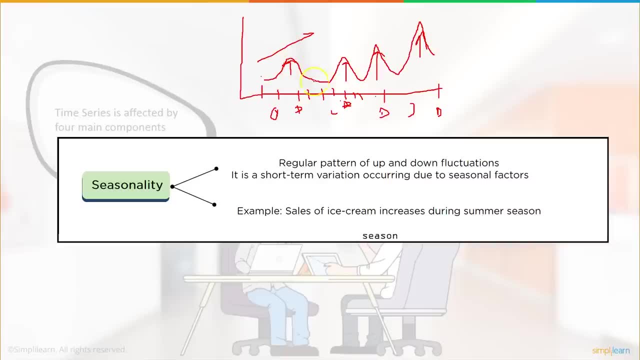 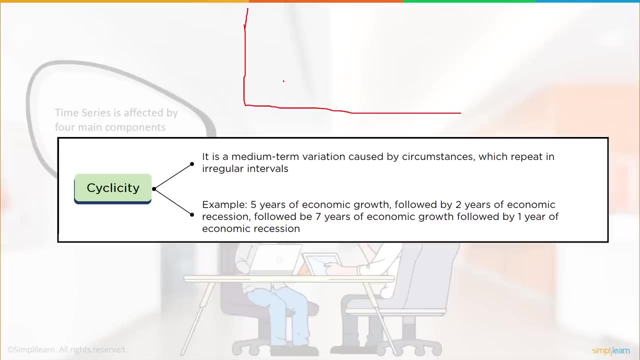 cycles is much longer. so seasonality typically is referred to as an annual kind of a sequence, like, for example, we saw here. so it is pretty much like every year in the month of december the sales are increasing. however, cyclicity. what happens is, first of all, the duration is pretty much not fixed, and the duration or the gap 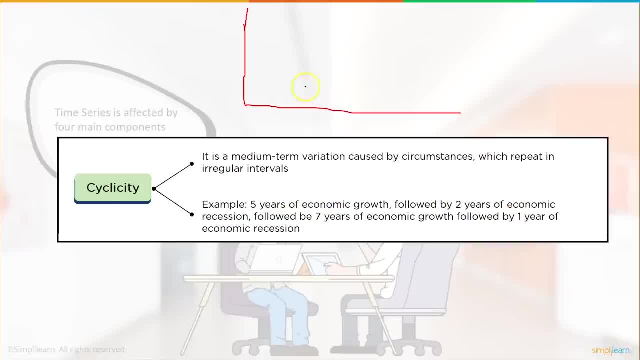 length of time between two cycles can be much longer. so recession is an example. so we had, let's say, recession in 2001 or 2002, perhaps, and then we had one in 2008, and then we had probably in 2000, 2012, and so on and so forth. so it is not like every year this happens, probably so. 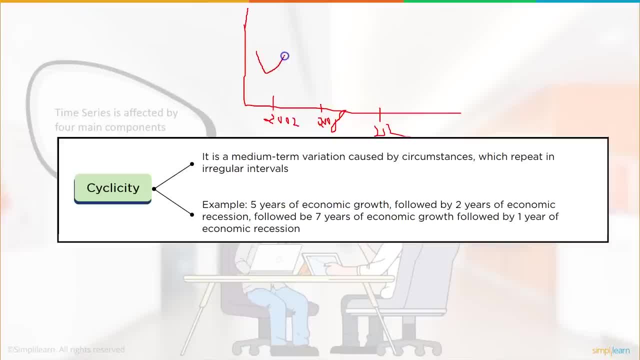 there is a- usually, when we say recession, there is a slump, and then it recovers, and then there is a slump and then it recovers, and probably there is another bigger slump, and so on. right, so you see, here this is similar to seasonality, but first of all, this length is much more than a year. right, that is. number one and it is not fixed as well. it is not like every four years or every six, perhaps seven or eight years it starts to rec restrictions. joy are w ten year in January being able to estimate the real weight loss figures and the total newspeda in the. in many cases this number is called its size. 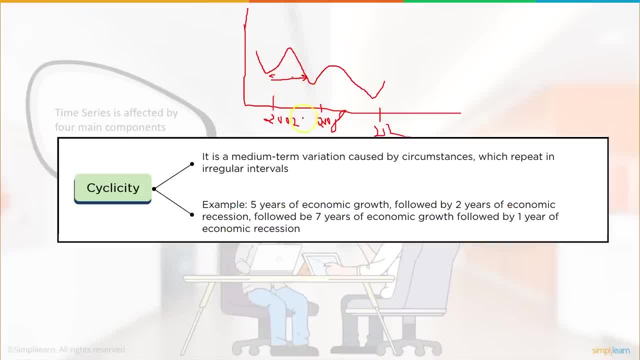 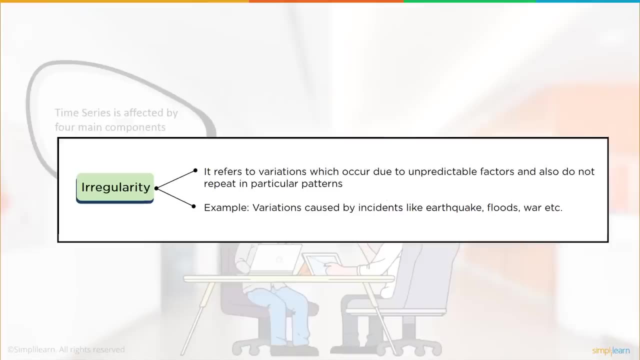 number one, and it is not fixed as well. it is not like every four years or every six years. that duration is not fixed, so the duration can vary. at the same time, the gap between two cycles is much longer compared to seasonality. all right, so then, what is irregularity? irregularity is like the 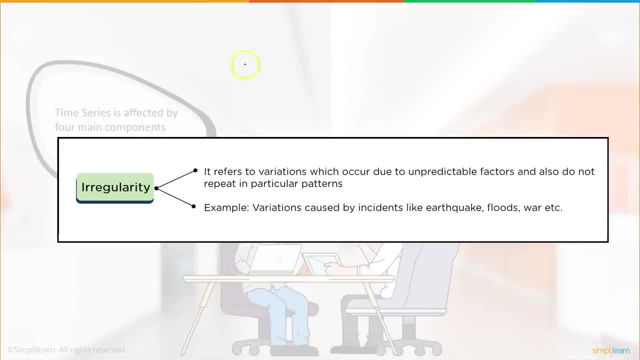 random component of the time series data. so there is, like you have part which is the trend, which tells whether the overall it is increasing or decreasing. then you have cyclicity and seasonality, which is like kind of a specific pattern. right, then there is a cyclicity, which is again a pattern. 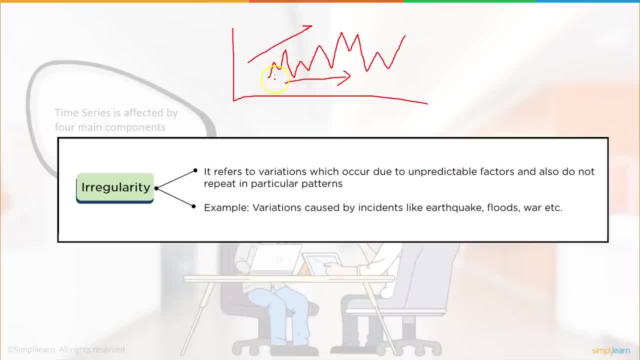 but at much longer intervals. plus, there is a random component, so which is not really, which cannot be accounted for very easily, right? so there will be a random component which can be really random, as the name suggests. right? so that is the irregularity component. so these are the various. 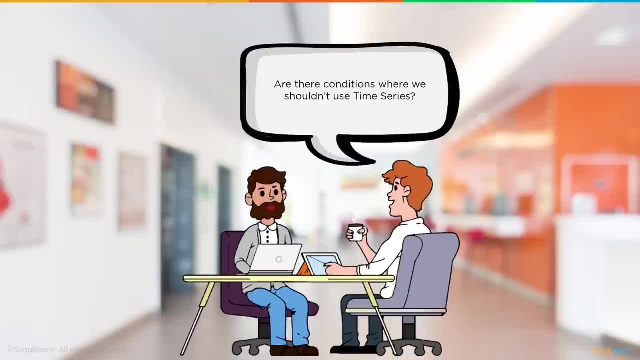 components of time series data, which is the one which is associated with the time series data series data. yes, there are conditions where we cannot use time series analysis. right so is it. can we do time series analysis with any kind of data? no, not really. so what are the situations? 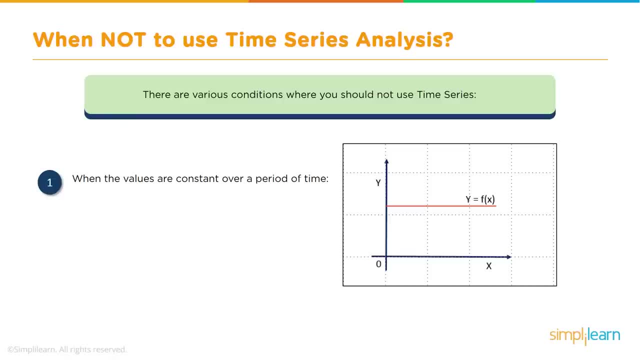 where we are, we cannot do time series analysis. so there will be some data which is collected over a period of time, but it's really not changing, so it will not really not make sense to perform any time series analysis over it, right, for example, like this one: so if we take x as the time and y 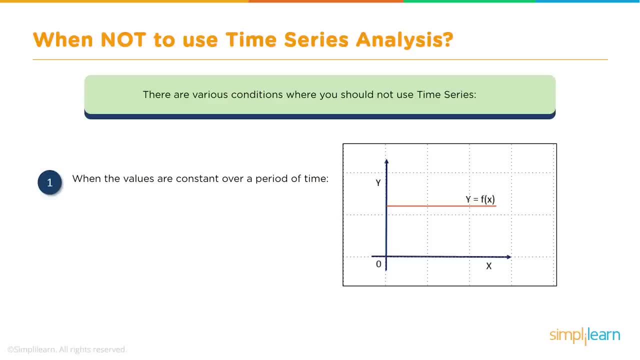 as the value of whatever the output we are talking about, and if the y value is constant, there is really no analysis that you can do, leave alone time series analysis, right? so that is one. another possibility is: yes, there is a change, but it is changing as per a very fixed function, like a sine. 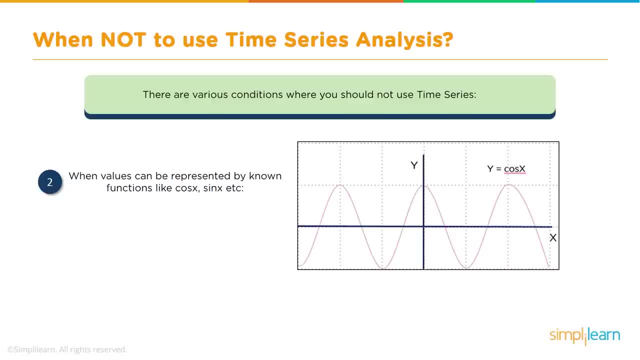 wave or a cross wave. again, time series analysis will not make sense in this kind of a situation, because if you wanted to do time series analysis with any kind of data, right, there are no time series analysis, right. so that is one. another possibility is: yes, there is a change, but it is. 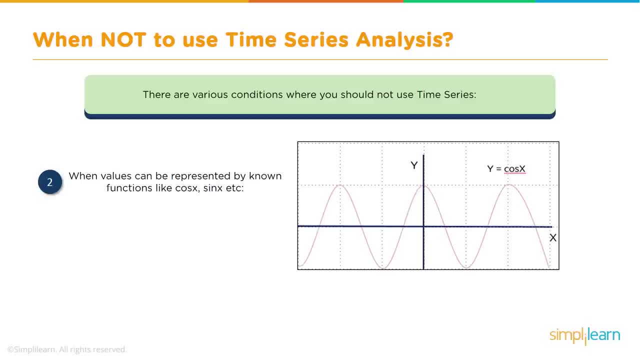 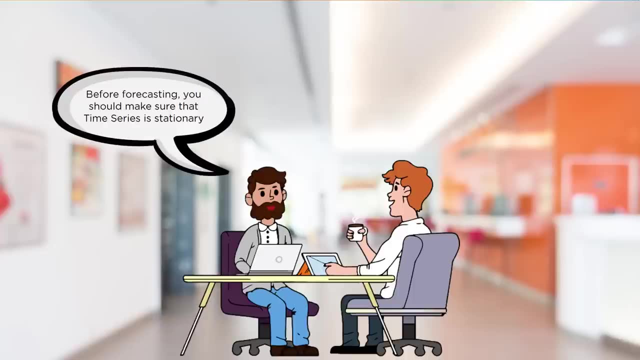 there is a definite pattern here. there is a definite function that the data is following, so it will not make sense to do a time series analysis now. before performing any time series analysis, the data has to be stationary and typically time series data is not stationary, so in which case you need to make the data stationary before we apply any models like. 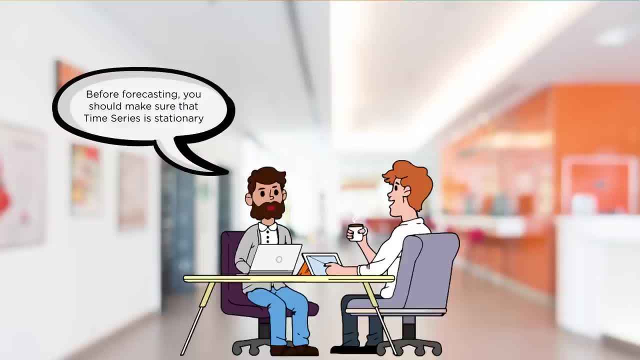 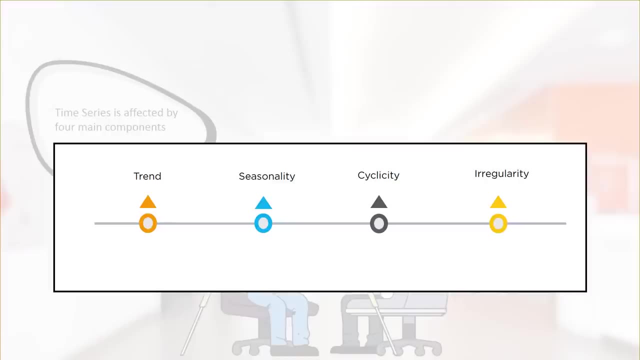 arima model or any of these, right? so what exactly is stationary data and what is meant by stationary data? let us take a look. first of all, what is non-stationary data? time series data. if you recall from one of my earlier slides, we said that time series data has the following four components: 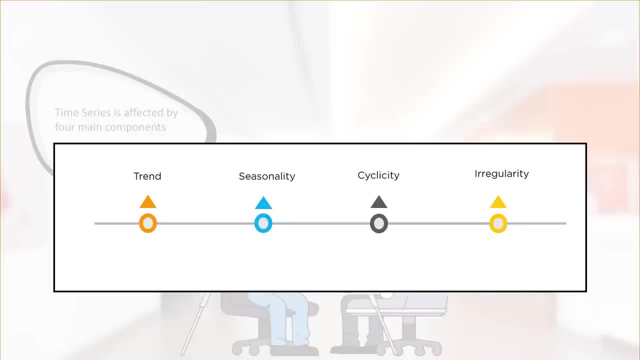 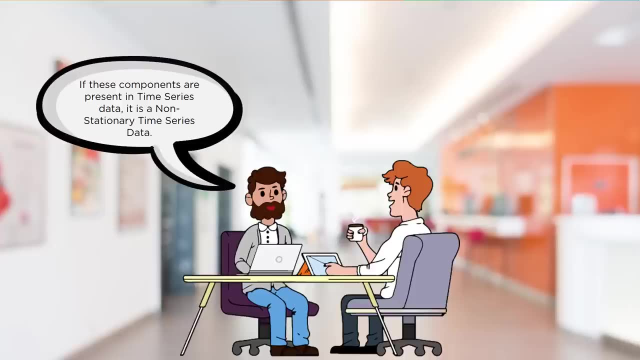 the trend, seasonality, cyclicity and random, random component or irregularity- right. so if these components are present in time series data, it is non-stationary, which means that you cannot solve a time series model of time series data using any of the above linked components. 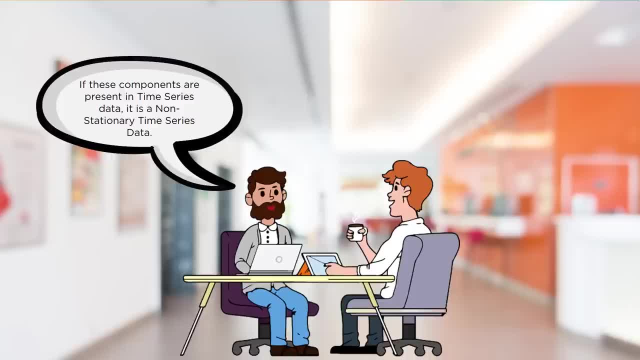 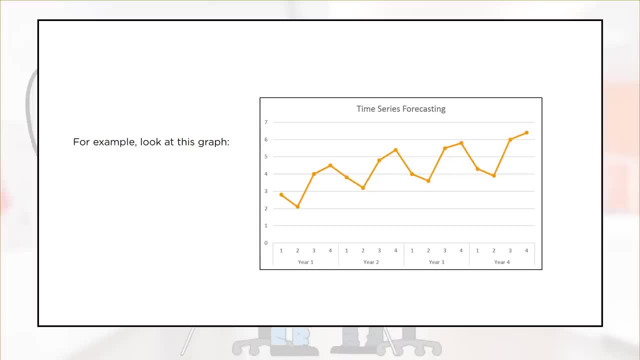 that typically these components will be present. therefore, most of the time, a time series data that is collected, raw data, is non-stationary data, so it has to be changed to stationary data before we apply any of these algorithms. all right, so a non-stationary time series data would look. 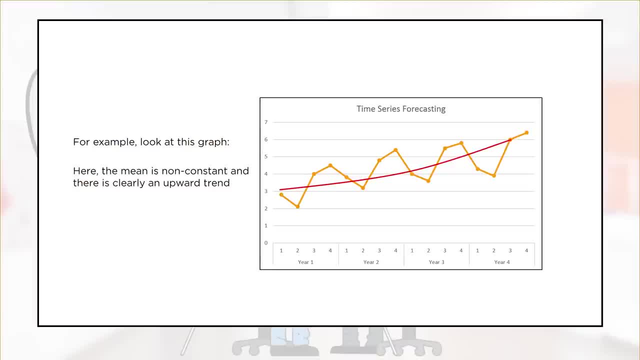 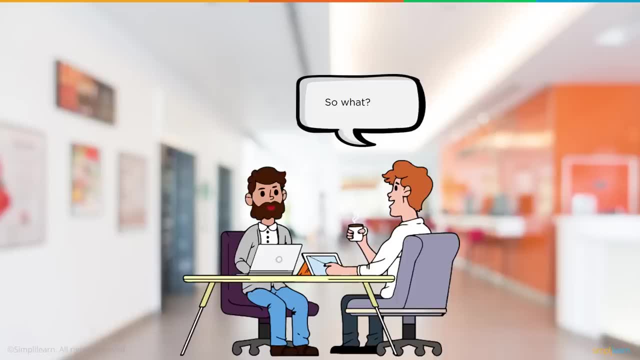 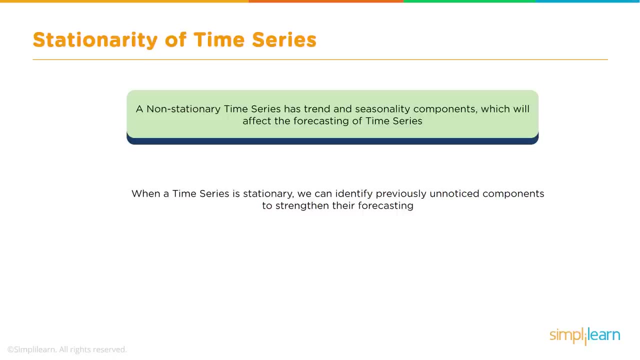 like this, which means like, for example, here there is an upward trend, the seasonality component is there and also the random component and so on. so if the data is not stationary, then that time series forecasting will be affected. so you cannot really perform a time series forecasting on a 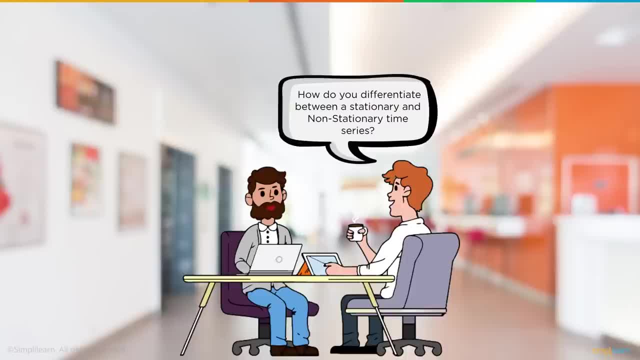 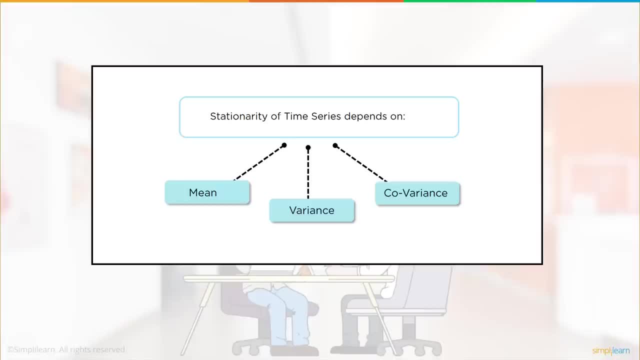 non-stationary data. so how do we differentiate between a stationary and a non-stationary time series data, typically or technically? one is, of course you can do it visually. in non-stationary data, the the data will be more flattish. seasonality will of course be there, but the trend will not be there, so the data may, if we plot that. 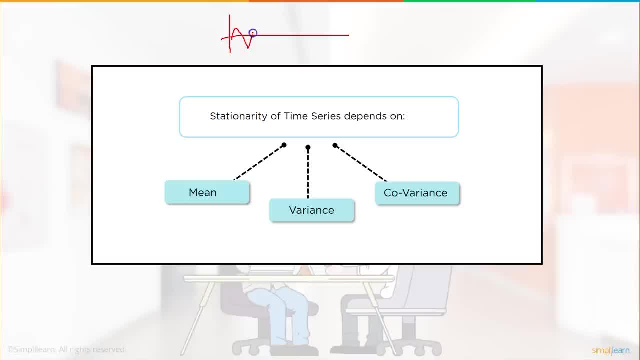 it may appear somewhat like this: right, it's a horizontal line. along the horizontal line, you will see, compared to the original data which was there was an upward trend, so it was changing somewhat like this right. so this is non-stationary data and this is how a stationary data would look. 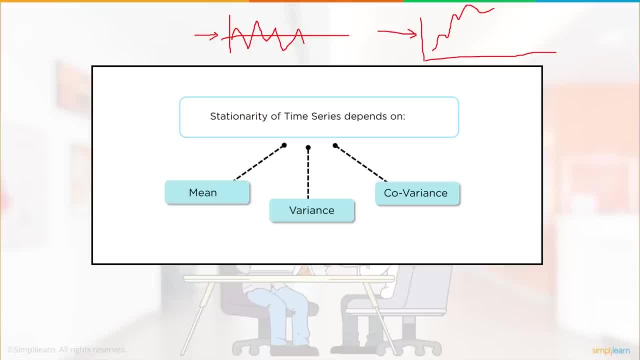 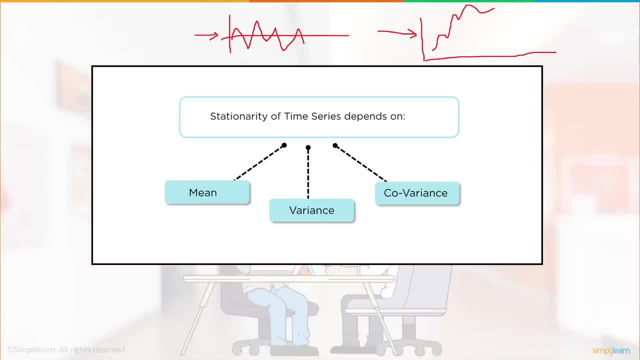 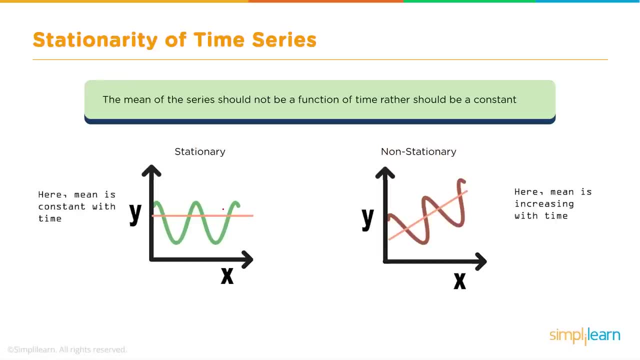 the mean, the variance and the covariance. so these are the three components on which the stationarity of the data depends. so let's take a look at what each of these are. for stationary data, the mean should not be a function of time, which means that the mean should pretty much 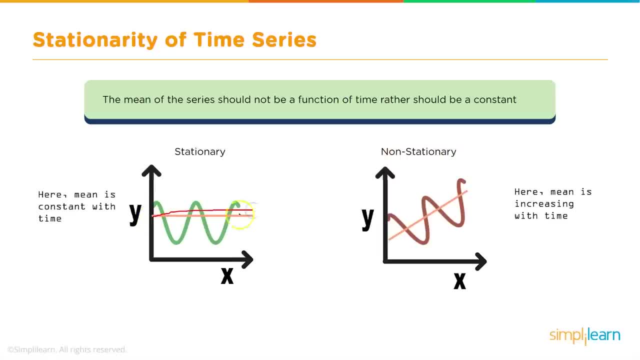 remain constant over a period of time. right, so there is, there shouldn't be any change. uh, so this is how the stationary data would look, and this is how a non-stationary data would look. i've shown in the previous slide as well. so here the mean is increasing. that means the mean is increasing. 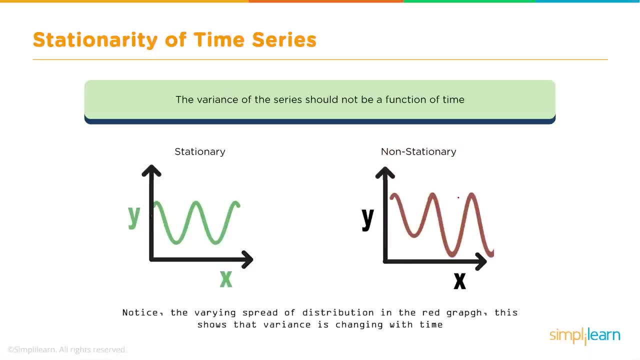 there is an upward trend. okay, so that is one part of it. and then the variance of the series should not be also a function of time, so the variance also should be pretty much common or should be constant, rather. so this is a if we visually, we take a look, this is how time series stationaries 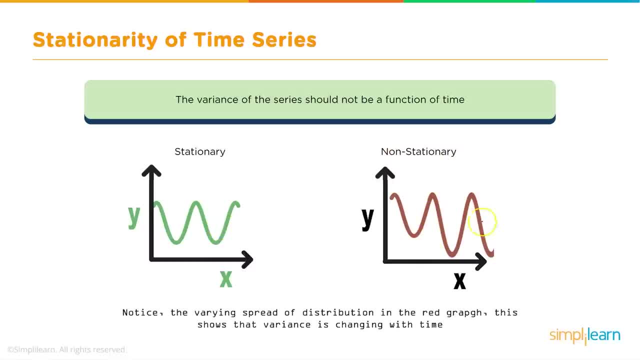 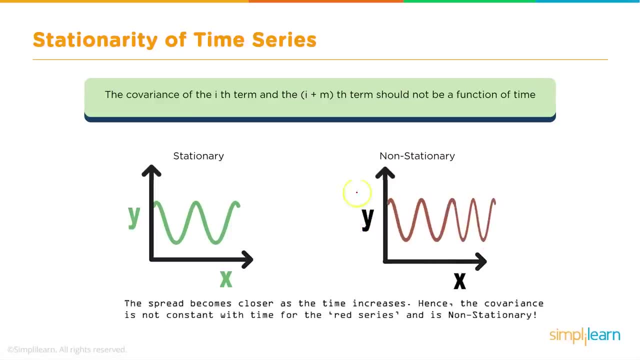 data would look where the variance is not changing. here the variance is changing. therefore, this is non-stationary and we cannot apply time series forecasting on this kind of data. similarly, the covariance which is basically of the ith term and the i plus mth term should not be a function of 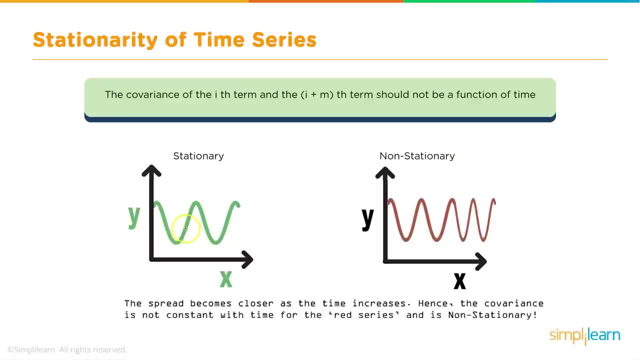 time as well. so covariance is nothing but not only the variance at the ith term, but the relation between the variance of the ith term and the i plus mth or the i plus nth term. so as again, once again, visually, this is how it would look if the covariance is also changing with respect to time. 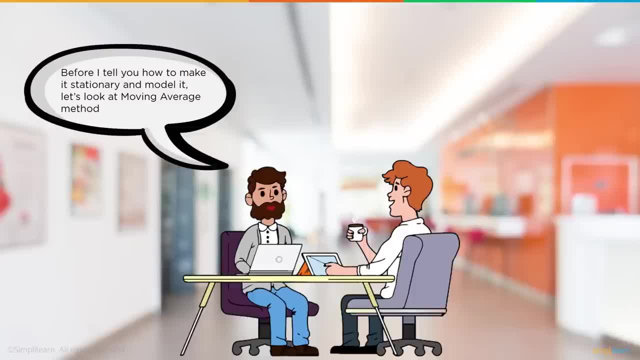 so these are the three. all three components should be pretty much constant, and that is when you have stationary data and in order to perform time series analysis, the data should be stationary. okay, so let's take a look at, uh, the concept of moving average or the method. 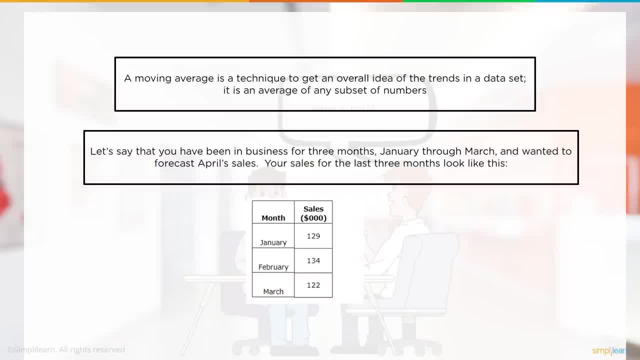 of moving average and let's see how it works. we'll do simple calculations, so let's say this is our sample data. we have the data for three months: january, february, march. the sales in hundreds of in thousands, rather not hundreds thousands of dollars is given here and 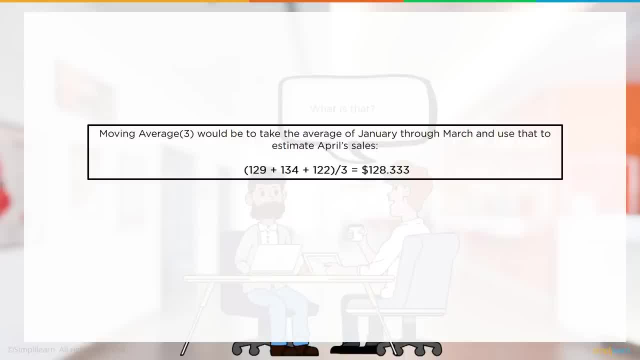 uh, now we want to find the moving average. so how do we find the moving average? we call it as moving average three. so moving average three is nothing, but you take three of the values or the readings, add them up and, uh, divide by three. basically the way we take a mean or. 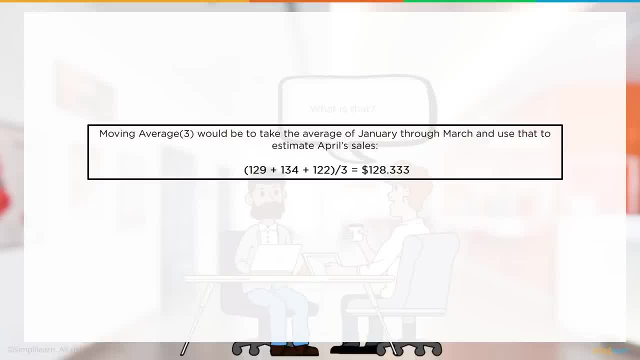 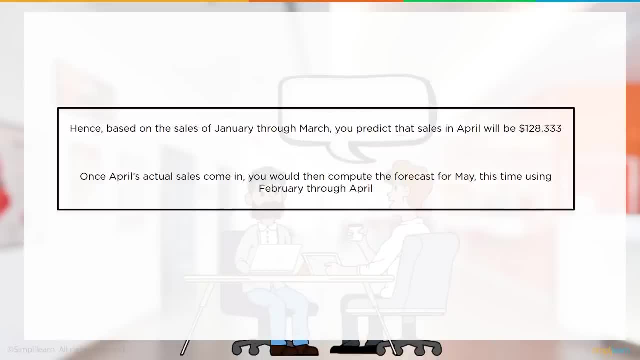 average of the three values. so that is as simple as that. so that's the average, first of all. so what is moving average? moving average is, if you now have a series of data, you keep taking the three values, the next three values, and then you take the average of that and then the next three. 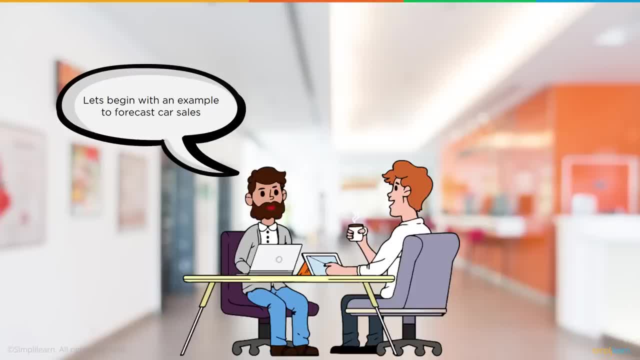 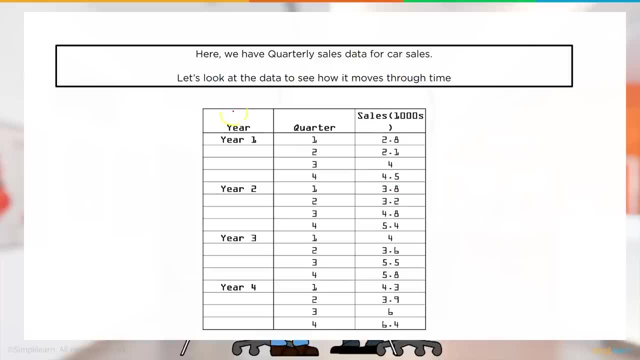 and so on and so forth. so that is how you take the moving average. so let's take a little more detailed example of car sales. so this is how we have the car sales data for the entire year- let's say so rather for four years. so year one we 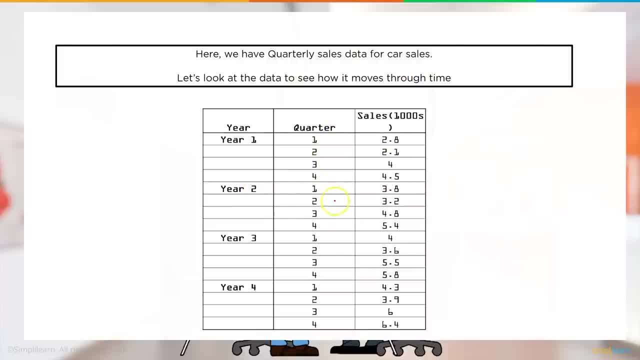 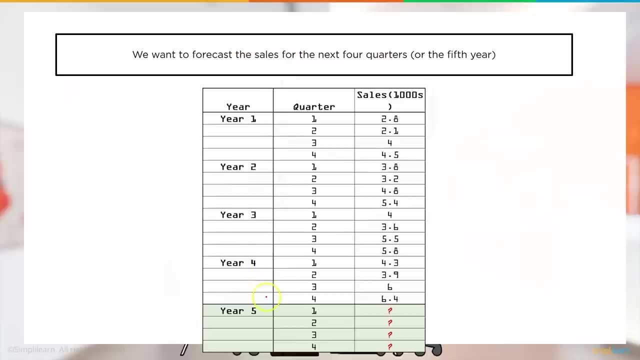 have for each quarter, quarter one, two, three, four, and then year two quarter one, two, three, four, and so on and so forth. so this is how we have sales data of particular car, let's say, or a showroom, and we want to forecast for year five. so we have the data for four years. we now want to focus for the fifth year, let's. 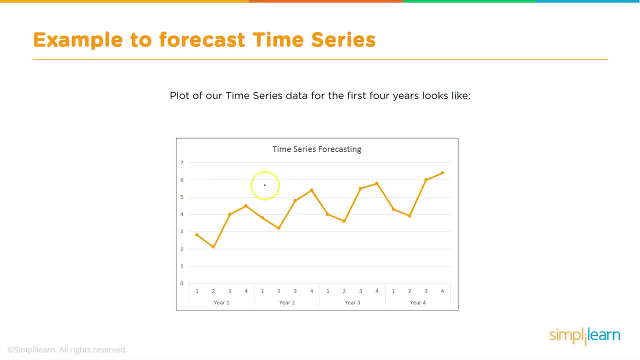 see how it works. first of all, if we plot the data as it is taken, the raw data, this is how it would look and what do you think it is? is it stationary? no right, because there is a trend, upward trend, so this is not a stationary data. 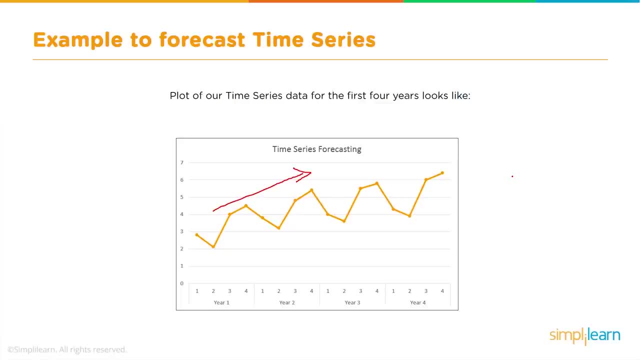 so we we need to. later we will see how to make it stationary, but to start with, just an example, we will not worry about it for now. we will just go ahead and manually you do the forecasting using what is known as moving average method. okay, so we are. 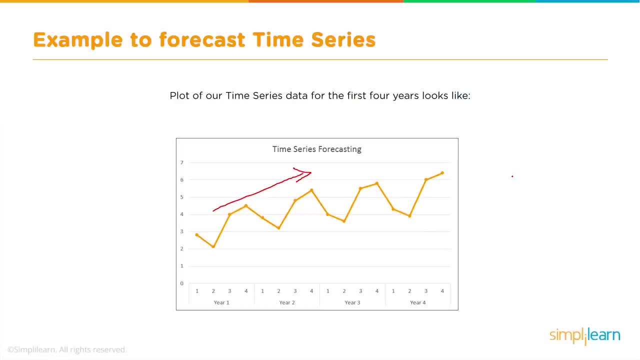 not applying any algorithm or anything like that. in the next video, we will see how to apply an algorithm, how to make it stationary, and so on. all right, so here we see that all the three or four components that we talked about are there. there is a trend, there is a seasonality and then, of course, there is 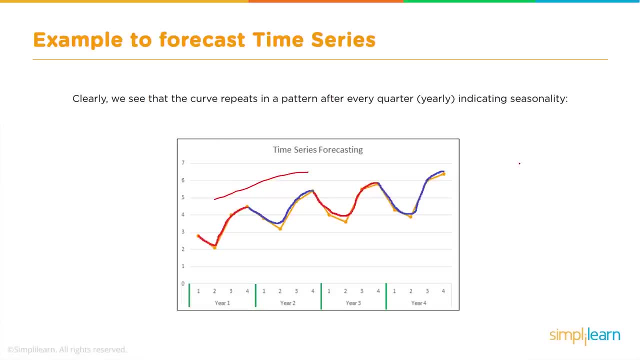 some random component as well, cyclicity may not be. it is possible that cyclicity is not applicable in all the situations for sale, especially. there may not be unless you are taking a sales for maybe 20, 30 years. cyclicity may not come into play. so we will just consider. 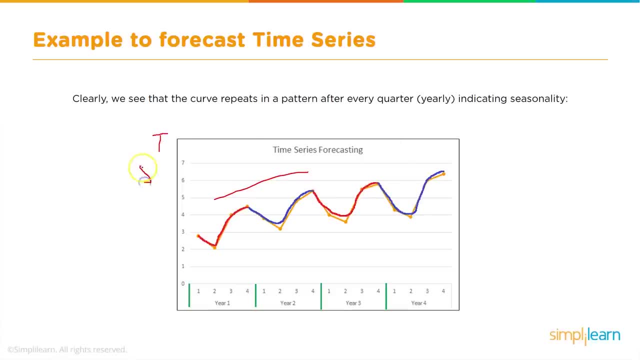 primarily the trend, seasonality and irregularity right. so random, it is also known as random irregularity right, so we were calling the random or irregularity component. so these are the three main components typically in this case we will talk about. so this is the trend component and 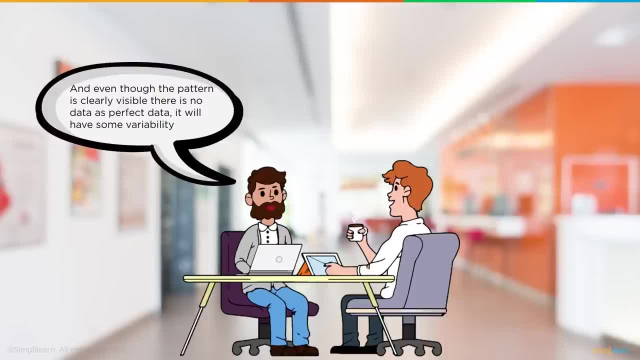 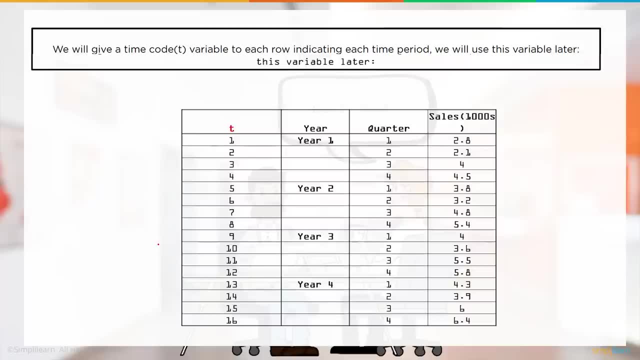 we will see how to do these calculations. so let's take a look. we draw the table including the time code. we will add another column, which is the time code, and it is the column, and we just number it like 1, 2, 3, 4, up to 16. the rest of the 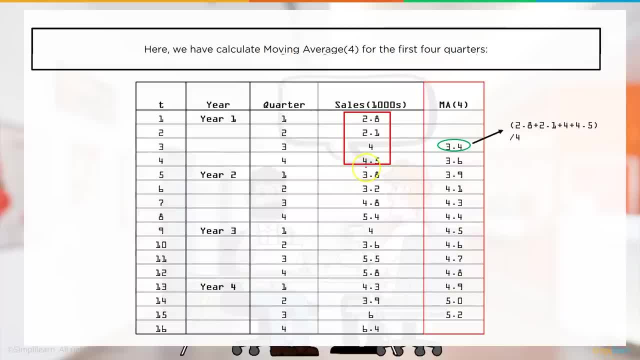 data remains the same. okay, so we will do the calculations now. now let us do the moving average calculations, or ma4 as we call it for each year. so we take all the four quarters and we take an average of that. so if we add up these four values, 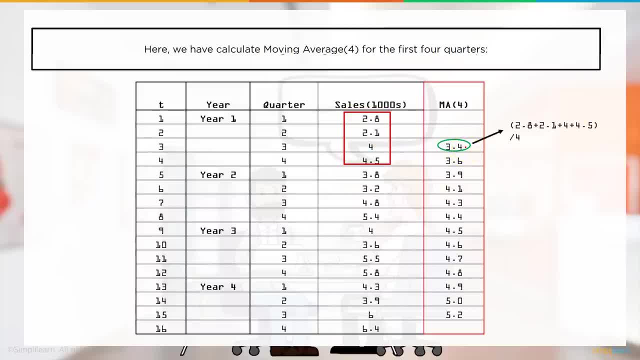 and divide by 4, you get the moving average of 3.4. so we start by putting the value here. so that will be for the third quarter. let's say 1, 2, 3, the third quarter, then we will go on to the next one. so we take the next four values, as you see here. 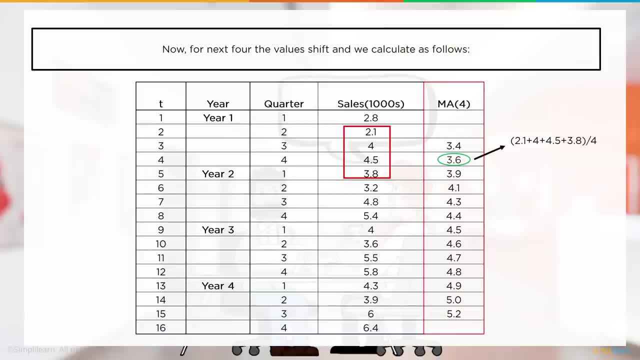 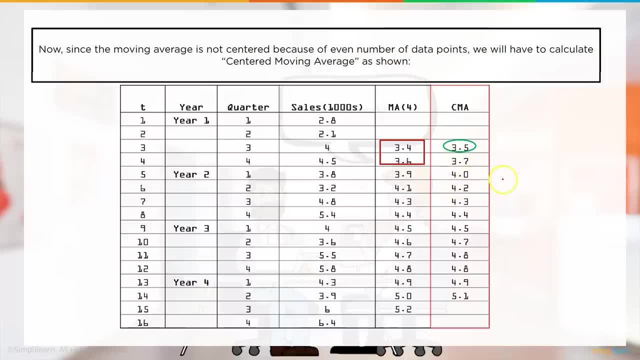 and take the average of that which is the moving average for the next quarter, and so on and so forth. we just do the moving average. it is not centered. so what we do is we basically add one more column and we calculate the centered moving average as shown here. so 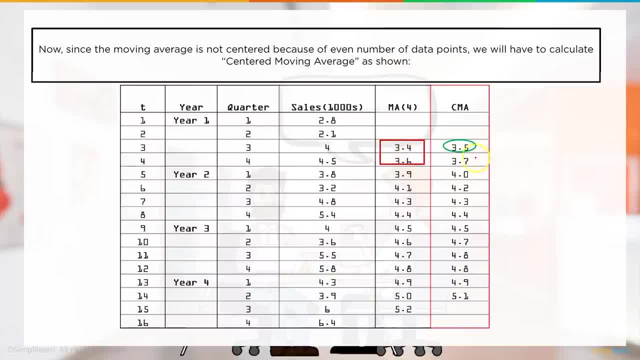 here. what we do is we take the average of two values and then just adding these values here. so, for example, the first value for the third quarter is actually the average of the third and the fourth quarter. so we have 3.5 now it gets centered. so, similarly, the next value would be 3.6 plus 3.9 divided by 2. so 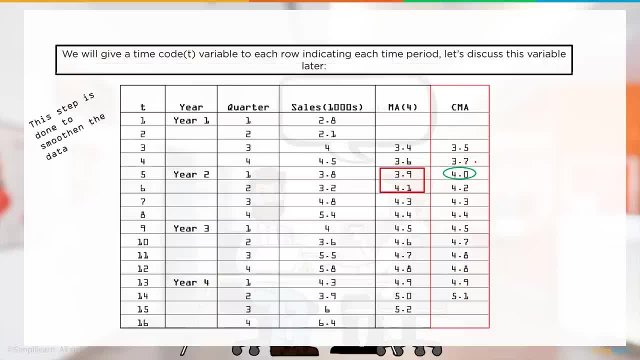 which is 3.7, and so on and so forth. okay, so that is the centered moving average. this is done primarily to smoothen the data so that there are not too many rough edges. so that is what we do here. so if we visualize this data now, this is how. 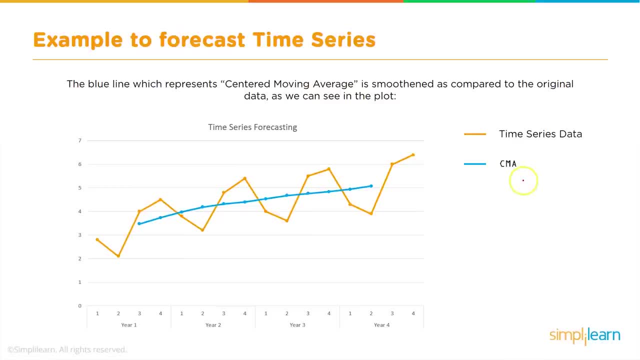 it looks right. so if we take the centered moving average, as you can see, there is a gradual increase. if we take the centered moving average, as you can see, this was not the case. if we had not centered it, the changes would have been much sharper. so that is the basically the smoothening that we are talking. 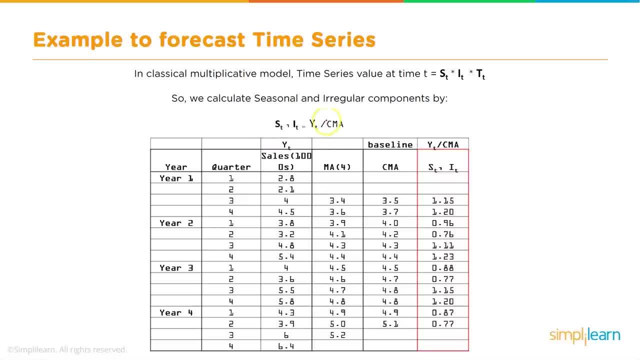 about now. let's go and do the forecast for the fifth year. so, in order to do the forecast, what we will do is we will take the centered moving average as our baseline and then start doing a few more calculations that are required in order to come up with the prediction. so what we are going to do is we are going to 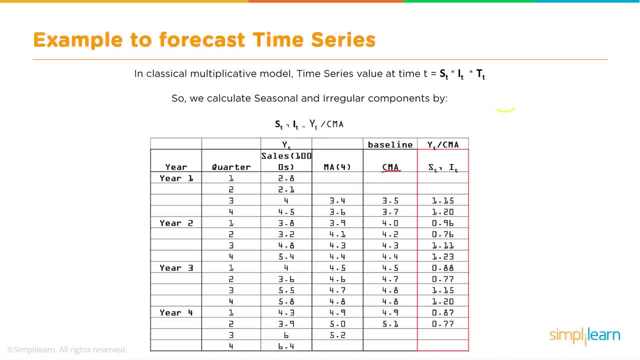 use this multiplicity or multiplicative model in this case, and this is how it it looks. so we take the product of seasonality and the trend and the irregularity components and we just multiply that and in order to get that, this product of these two, we have. 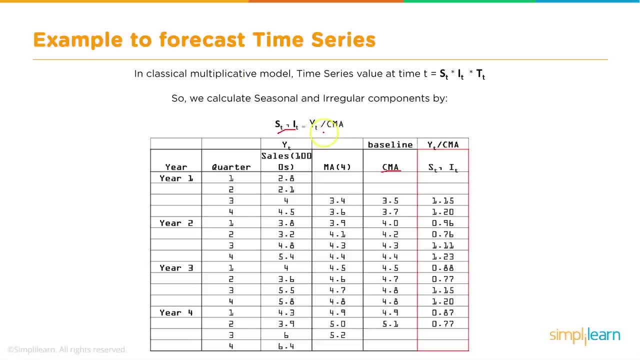 basically the actual value divided by cma. yt value divided by cma will give you the predicted value of yt is equal to the product of all three components. therefore, st into it is equal to yt by cma. so this is like: this is equal to yt. 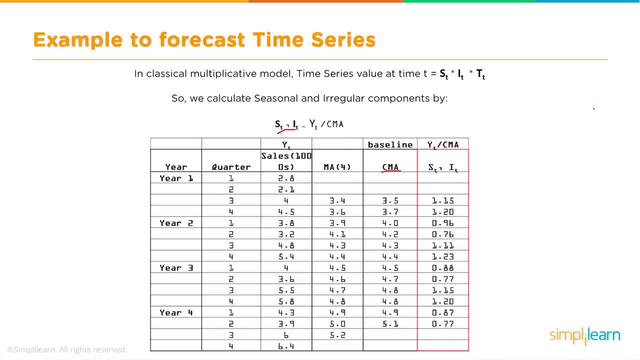 right. so therefore, if we want st into it, the product of seasonality and irregularity, it is equal to yt by cma. so that is how we will work it out. i also have an excel sheet of the actual data, so let me just pull that up. all right, so? 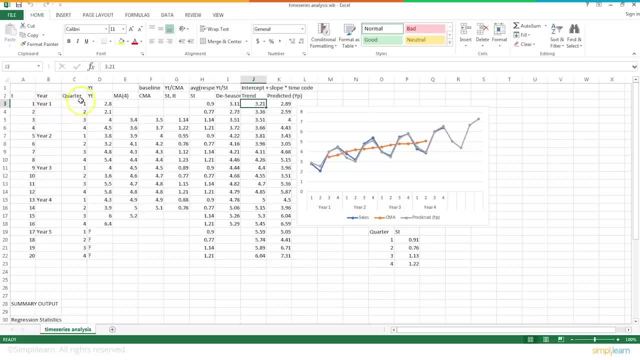 this is how the data looks in excel, as you can see here: year one quarter one, two, three, four. year two quarter one, two, three, four, and so on, and this is the sales data, and then this is the moving average. as i mentioned, this is how we calculate and this is the centered moving average. 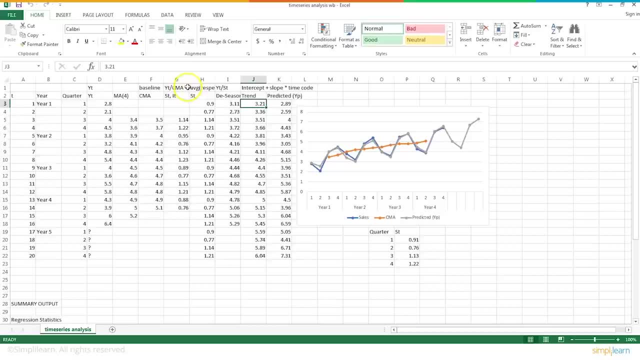 so this is the primary component that we will start working with and then we will calculate, since we want the product of st into it. that is equal to yt by cma. so, if you see, these values are nothing but the yt value divided by cma. so in this case it is 4 by 3.5, which is 1.14. similarly, 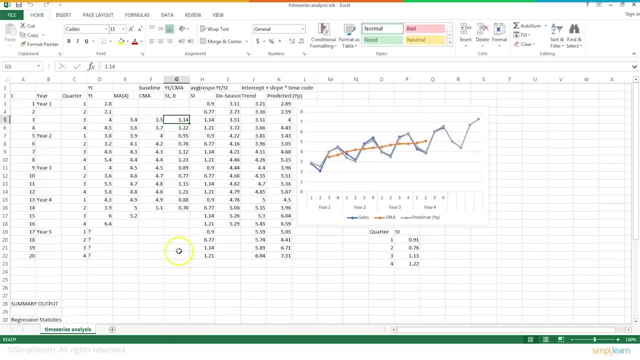 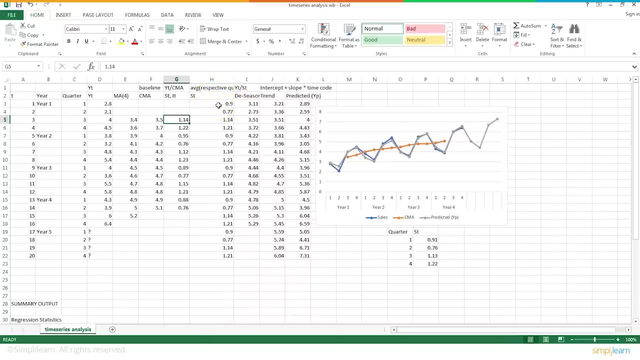 4.5 by 3.7, 1.22 and so on and so forth. so we take, we have the product st into it, and then the next step is to calculate the average of respective quarters. so that is what we are doing here: average of respective quarters. and then we need to calculate the de-seasonalized values. so in 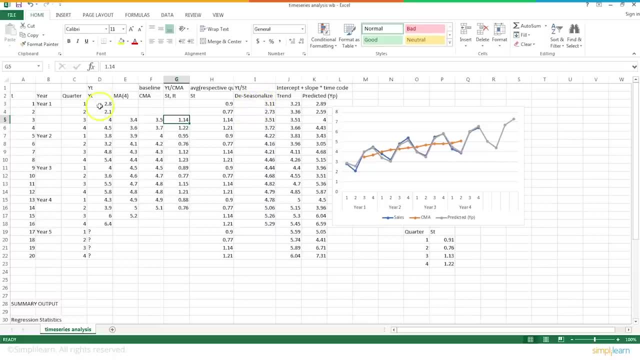 order to get de-seasonalized value, we need to divide yt by st. that was calculated. so, for example, here it is 2.8 by 0.9. so we got the de-seasonalized value here and then we get the trend and then we get the predicted values. so in order to get the predicted value, which is 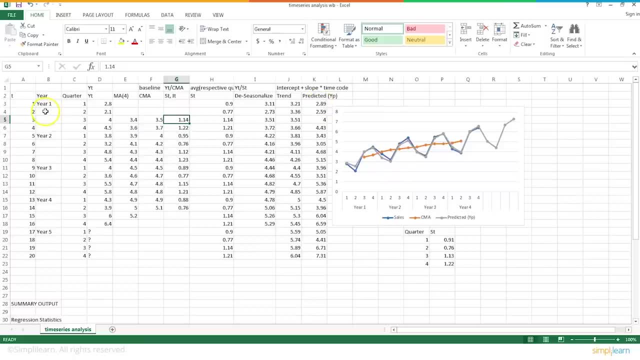 basically, we predict the values for known values as well, like, for example, year one quarter one. we know the value, but now that we have our model, we predict ourselves and see how close it is. so we predict it as two point eight nine, whereas the actual value is two point eight. and then we get. 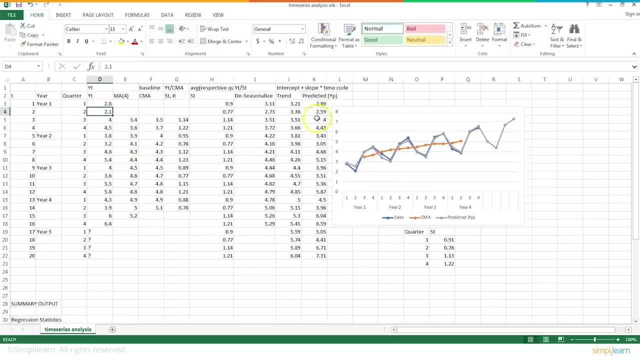 then we have 2.59, the actual value is 2.1, and so on, just to see how our model works, and then continue that into the fifth year, because in for fifth year we don't have a reference value. okay, and if we plot this we will come to know how well our calculations are, how well our manual. 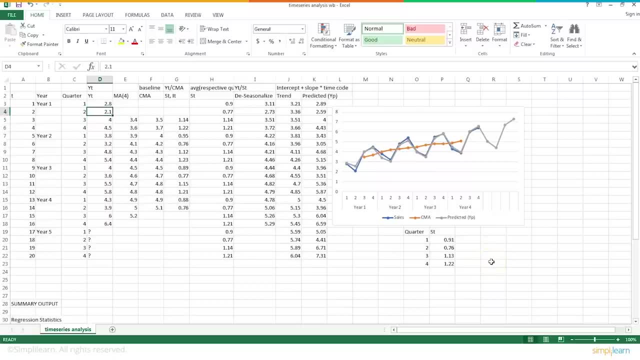 model. in this case we did not really use a model, but we did on our own, manually, so it will tell us the trend. so, for example, the predicted value is this gray color. here you can see that it is actually pretty much following the actual value, which is the blue. 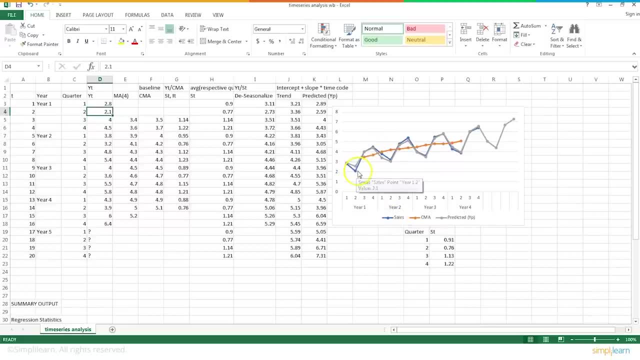 color right, and the gray color is the predicted value. so the wherever we know the values up to year four, we can see that our predicted values are following, or pretty much very close to the actual values. and then from here onwards, when the year five starts, the blue color. 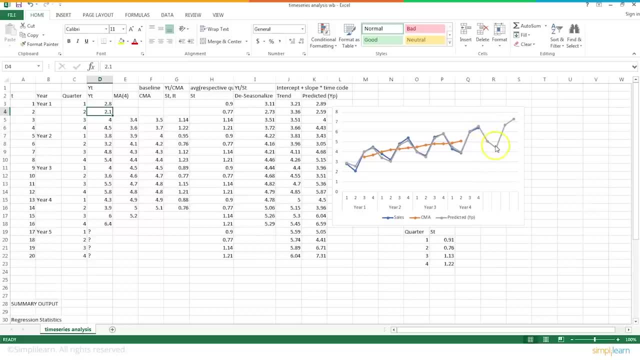 line is not there because we don't have the actual values, only the predicted value. so we can see that, since it was following the trend pretty much for the last four years, we can safely assume that it has understood the pattern and it is predicting correctly for the. 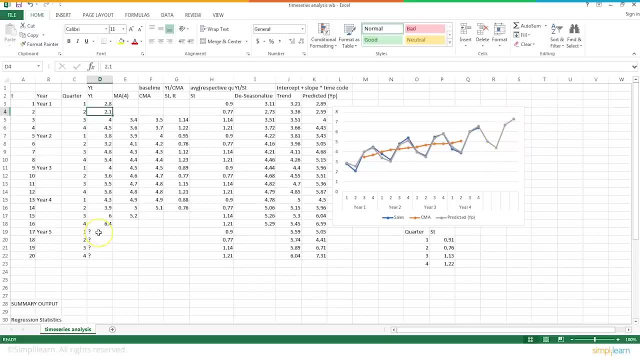 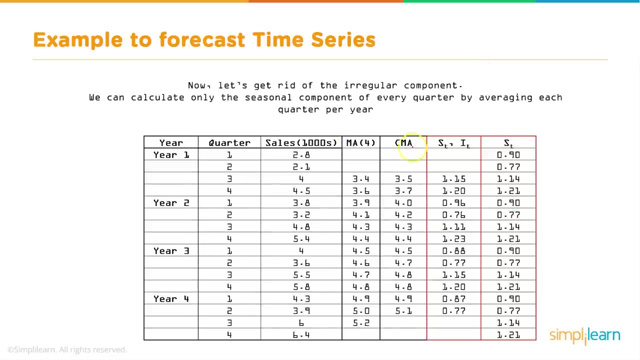 next one year, the next four quarters, right, so that is what we are doing here. so these four quarters we did not have actual data, but we have the predicted values. so let's go back and see how this is working in this using the slides. so this is. we already saw this part and i think it was. 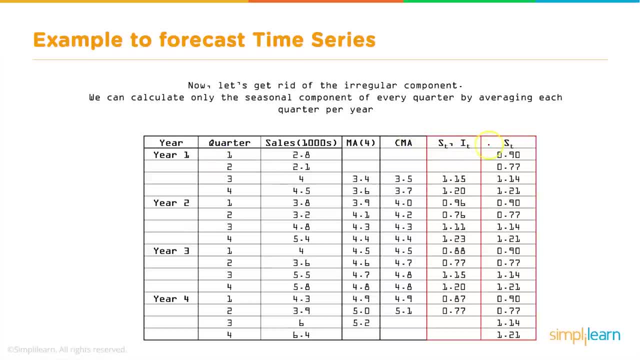 easier to see in the excel sheet. so we calculated the st, it, the product of st, and it using the formula like here: y by yt, by cma. we got that and then we got st, which is basically yt. so this is the average of the first quarters for all the four years and similarly this is the average of. 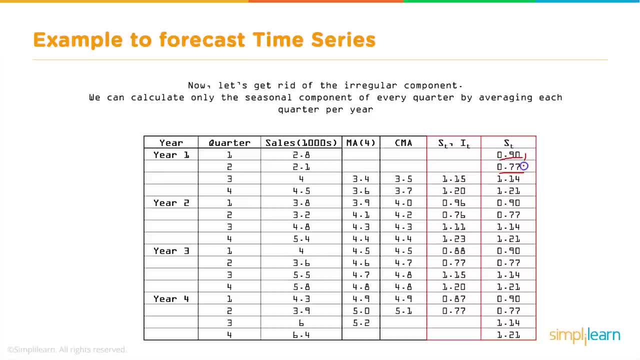 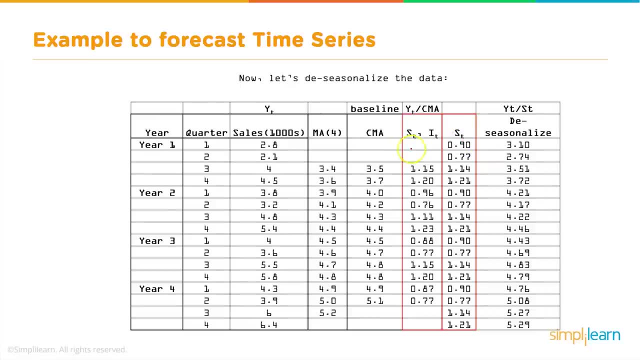 the second quarter, for all the four years and so on. so these values are repeating. these are. they are calculated only once. they get repeated, as you can see here, and then we get the de-seasonalized data and that is basically yt by st. so we calculated st here and we have yt, so yt by st will give you the de-seasonalized data. 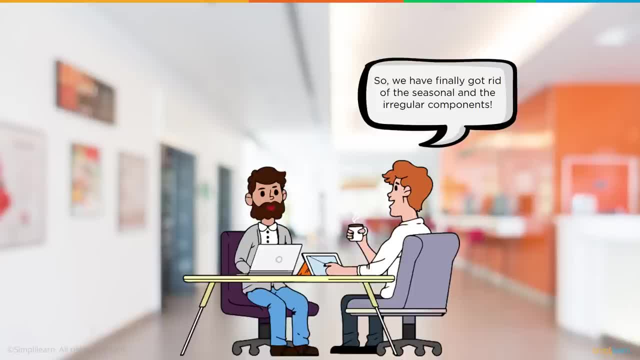 and we have got rid of the seasonal and the irregular components so far. now what we are left with is the trend, and before we start the time series forecasting or time series analysis, as i mentioned earlier, we need to completely get rid of the non-stationary. 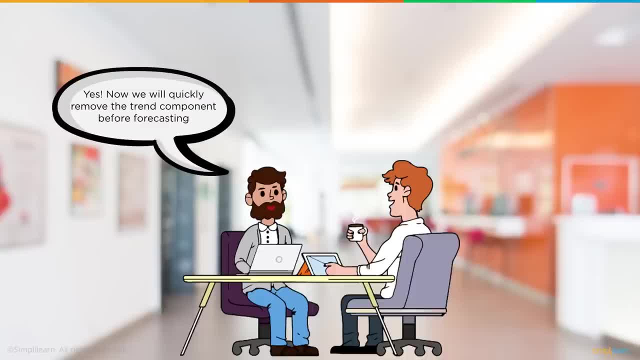 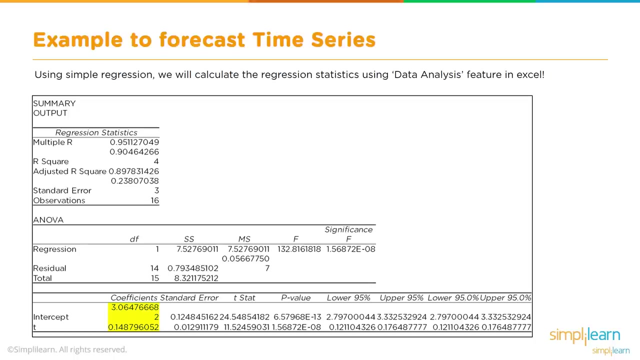 components. so we are still left with the trend component. so now let us also remove the trend component. in order to do that, we have to find the, or we have to calculate the intercept and slope of the data, because that is required to calculate the trend. and how are we going to do that? we will actually use what is known as a regression tool or analytics. 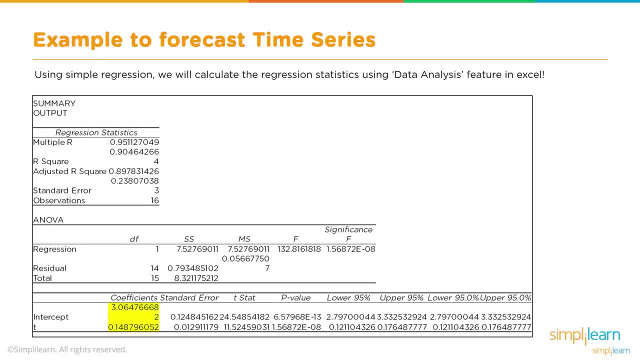 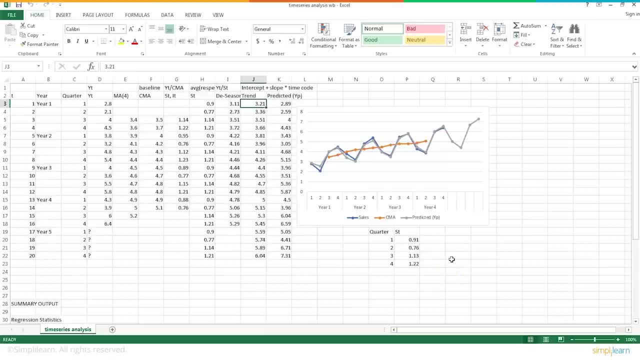 tool that is available in excel. so you remember, we have our data in excel. so let me take you to the excel, and here we need to calculate the intercept and the slope. in order to do that, we have to use the regression mechanism, and in order to use the regression mechanism, we have to use the analytics. 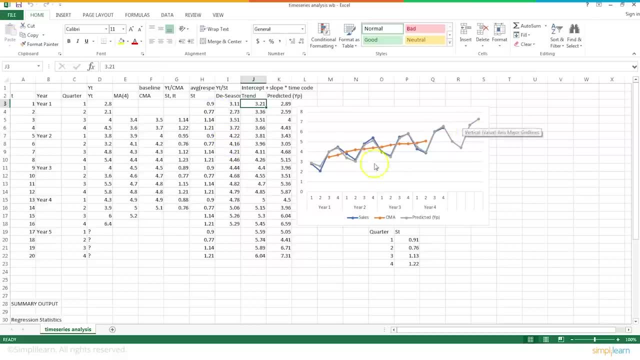 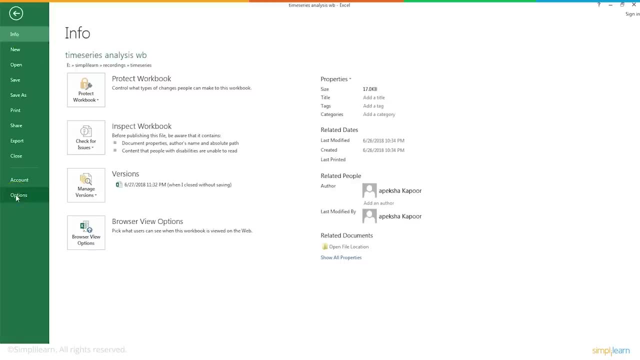 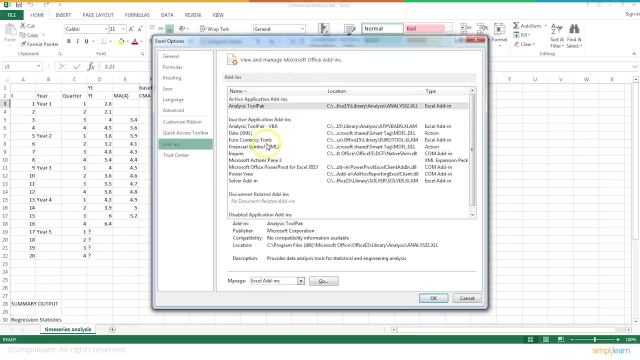 tool that comes with excel. so how do you activate this tool? so this is how you would need to activate it. so in excel, you need to click on the data tool in excel toolpacks. and when we click on the data tool from excel, you need to go to options, and in options there will be add-ins and in add-ins you. 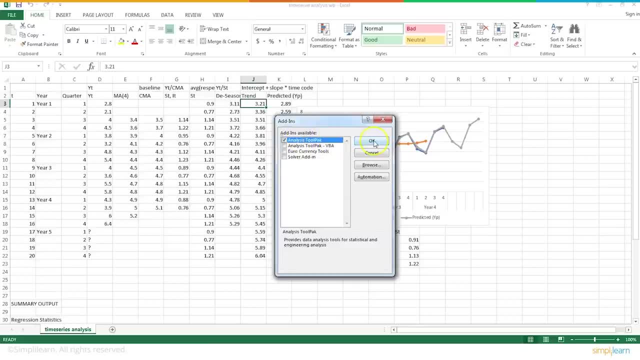 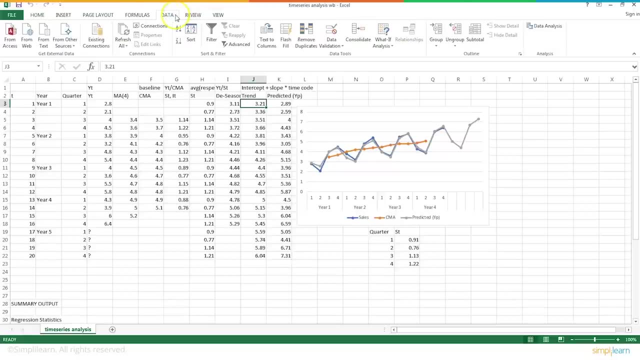 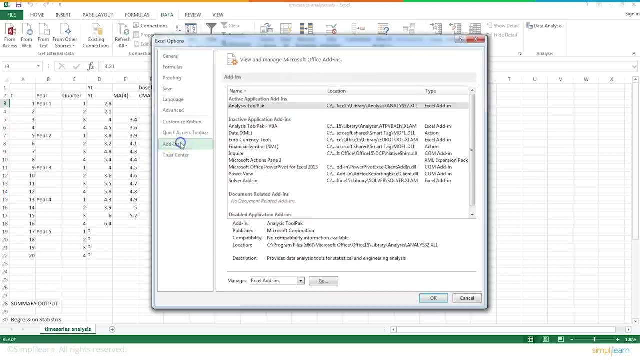 will have analysis tool back and you select this and you just say go. it will open up a box like this. you say analysis tool pack and you say okay, and now data tab. you will see data analysis activated. so you need to go to file options and add-ins and 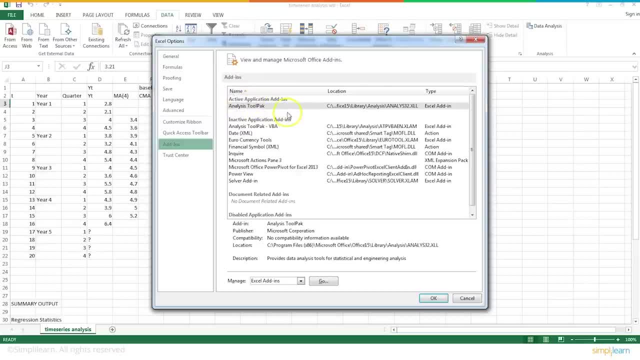 then analysis tool pack. typically, since I've already added it, it is coming at the top, but it would come under inactive application add-ins. so when you're doing it for the first time, so don't use VBA, you just say analysis tool pack. there are two options: one with VBA, like this: 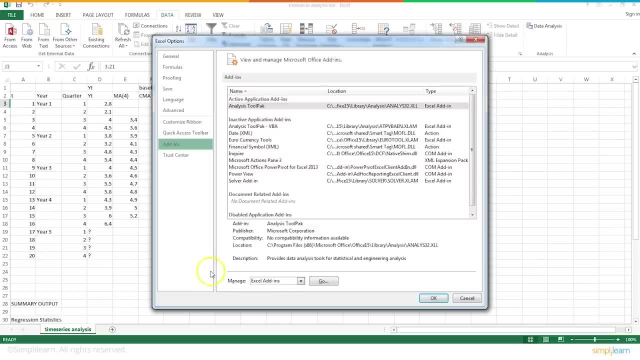 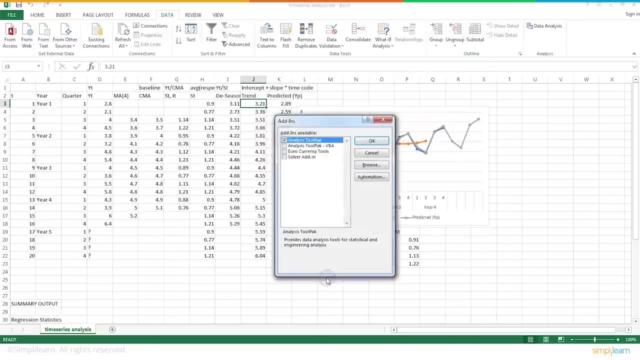 one and one without VBA. so just use the one without VBA. and then, instead of just saying okay, just take care that you click on this go and not just okay. so you say go, then it will give you these options. only then you select just the analysis tool pack and then you say: okay, all. 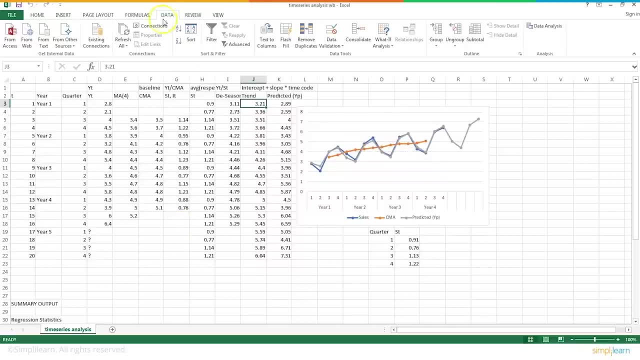 right, so, and then, when you come back to the main view, you click on data. okay, so this is your normal home view, perhaps. so you need to come to data, and here is where you will see data analysis available to you, and then, if you click on that, there are a bunch. 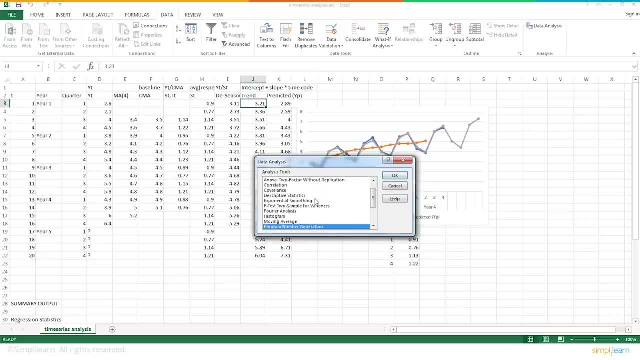 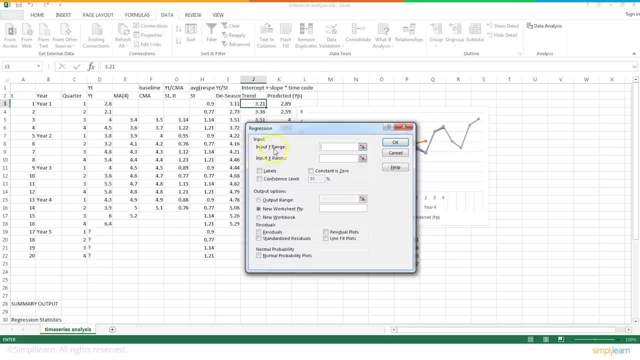 of possibilities? what kind of data analysis you want to do if there are options are given right now we just want to do regression because we want to find the slope and the intercept. so select regression and you say okay, and you will get these options for input y range and input x range. input. 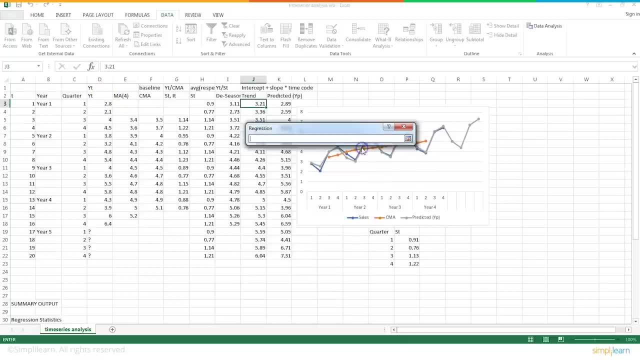 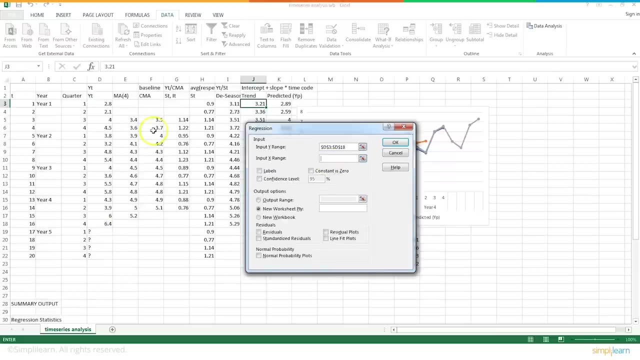 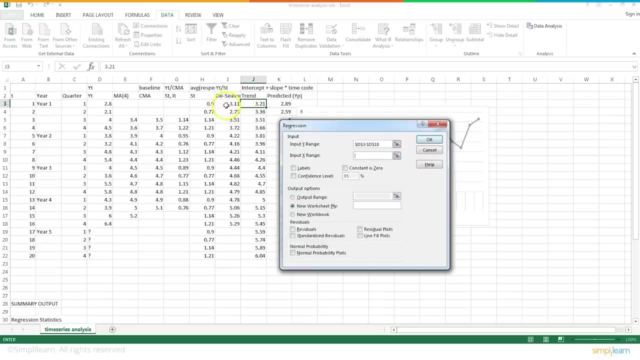 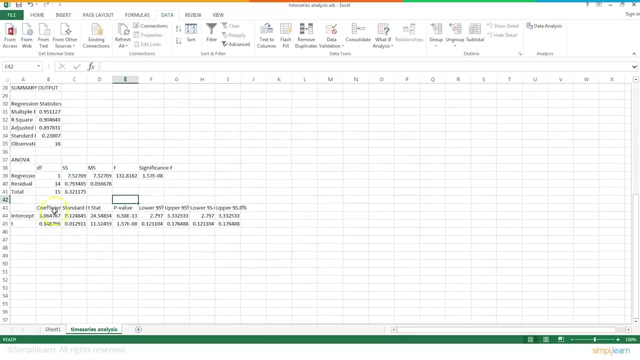 y range is the value yt. so you just select this and you can select up to here and press enter and input x range. you can, for now you start with the baseline, or you can also start with the de-seasoned values, so you can just click on these and say, okay, I have already calculated it. so these are the intercept and the coefficients. 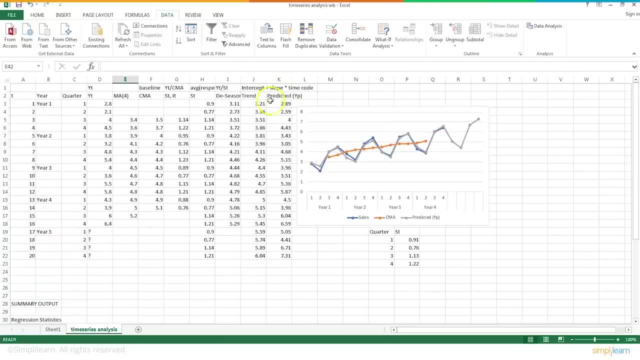 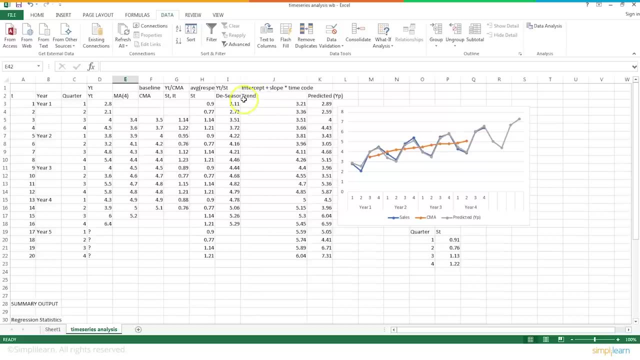 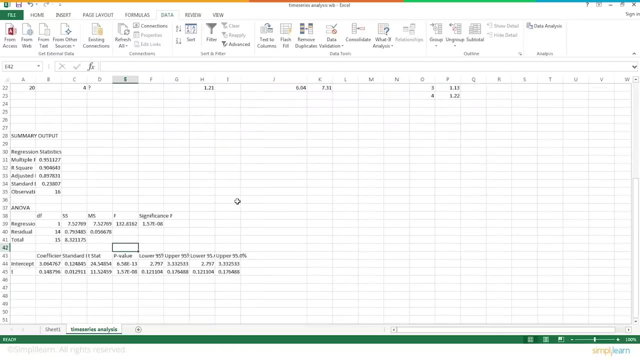 that we are getting for these values and we will actually use that to calculate our trend here. right so, which is in the J column? so our trend is equal to intercept plus slope into the time code. so the intercept is uh out here, as we can see in our slide as well. so if you see here, 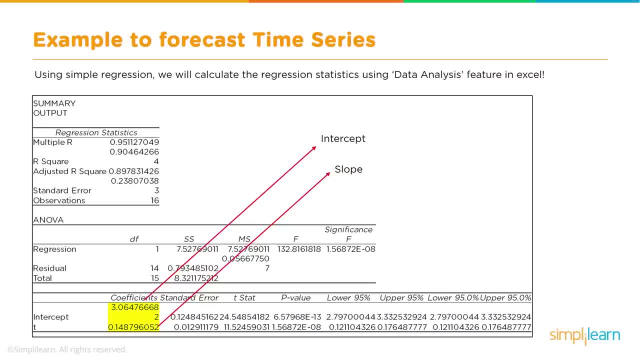 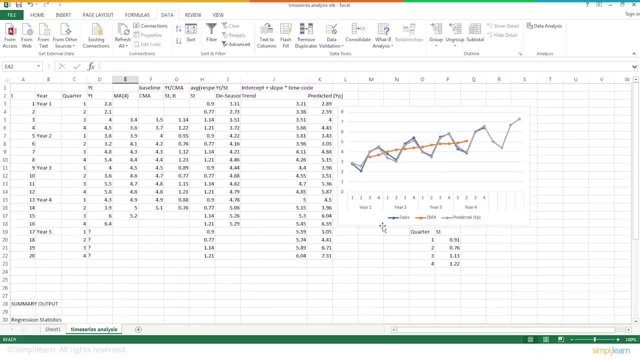 this is our intercept, and the lower value is the slope. so we have calculated here and it's shown in the slides as well. so intercept, so the formula is shown here. so our trend is equal to intercept, plus into time code. time code is nothing but this one, T, column a. one, two, three, four. okay, so that's how. 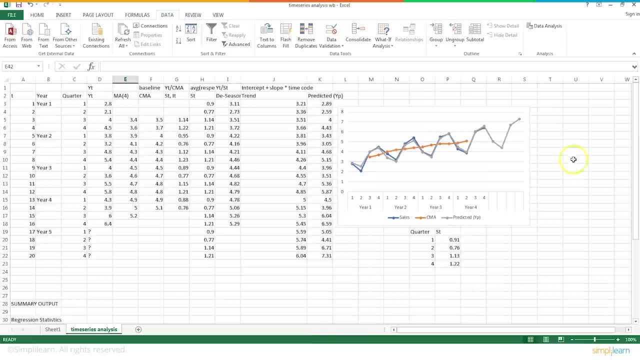 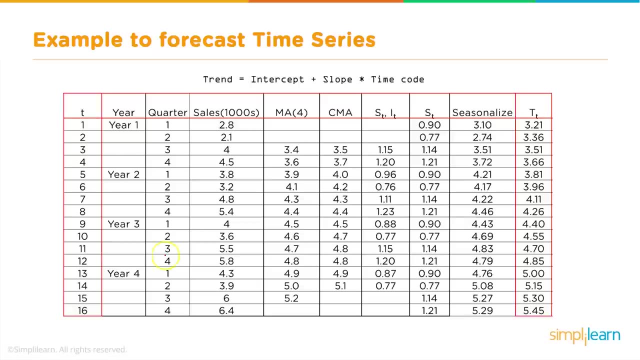 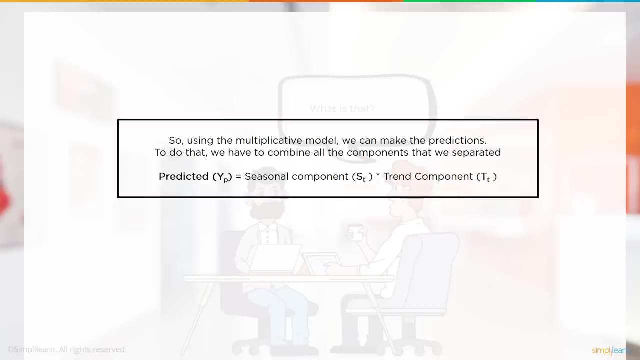 you calculate the trend and that's how you use the data analysis tool from Excel. using these two, we calculate the predicted values and using this formula, which is basically trend, is equal to intercept plus slope into time code, and then we can go and plot it, see how it is looking and 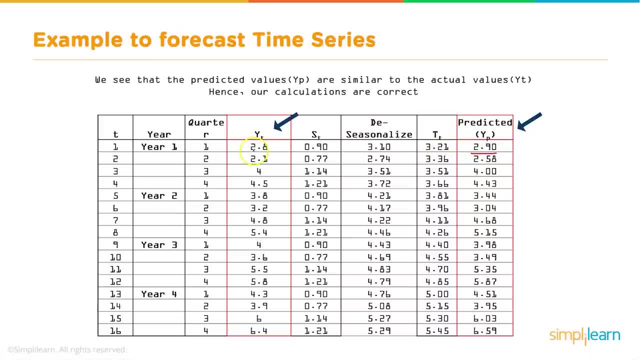 therefore. so we see here that the predicted values are pretty close to the actual values and therefore we can safely assume that our calculations, which are like our manual model, is working. and hence we we go ahead and predict for the fifth year, so till four years. we know the actual value as well, so we can compare our model. 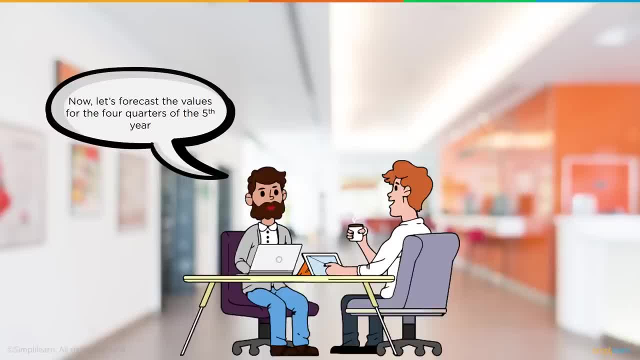 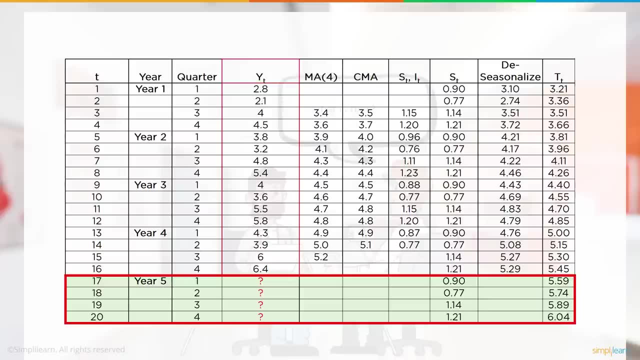 is performing and for the fifth year we don't have reference values. so we can use our equations to calculate the values or predict the values for the fifth year and we can go ahead and safely calculate those values and when we plot for the fifth year as well. the 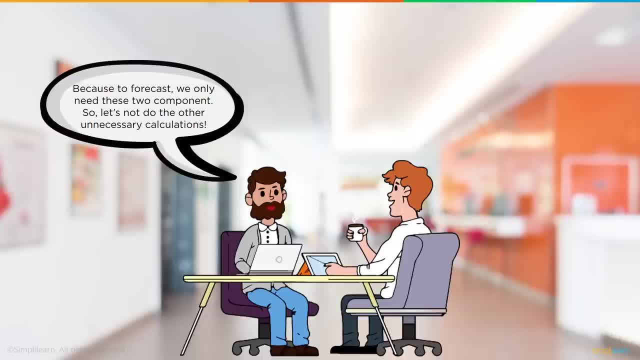 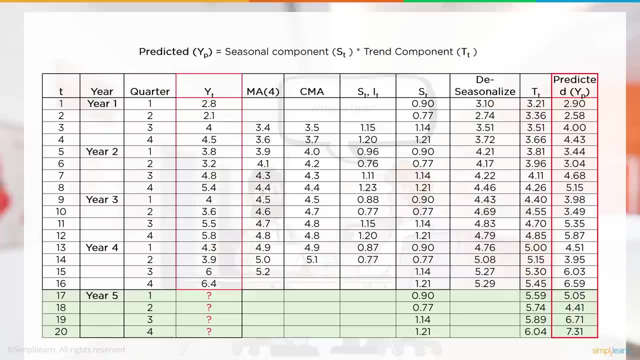 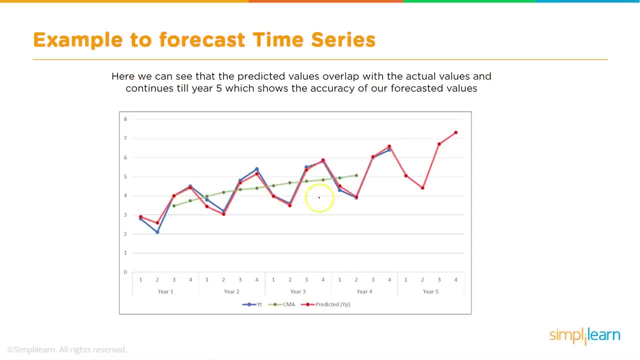 predicted values. we see that they are pretty much. they capture the pattern and we can safely assume that the predictions are fairly accurate, as we can also see from the graph in the Excel sheet that we have already seen. okay, so let's go and plot it. so this is how the plot looks. this is: 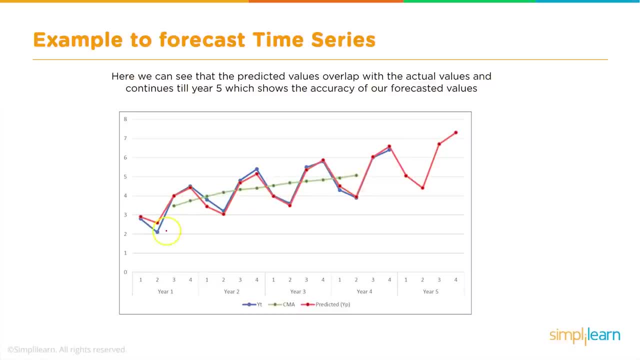 the CMA or the centered moving average, the green color and then the blue color, the actual data. red color is the predicted value predicted by our handcrafted model. okay, so remember we did not use any regular forecasting model or any tool. we have done this manually and the actual 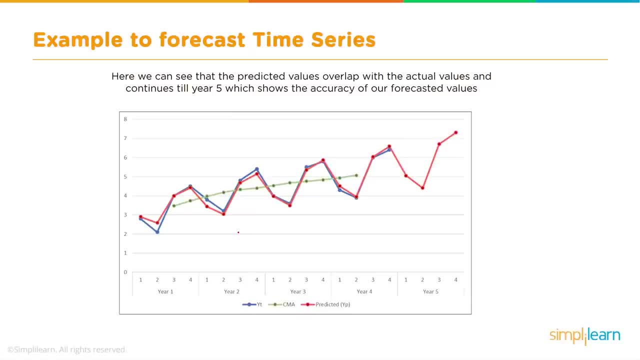 tool will be used in the next video. this is just to give you an idea about how, behind the scenes, or under the hood, how forecasting works. a time series analysis, how it is performed. okay, so it looks like it has captured the trend properly. so up to here is the known reference. we have reference. 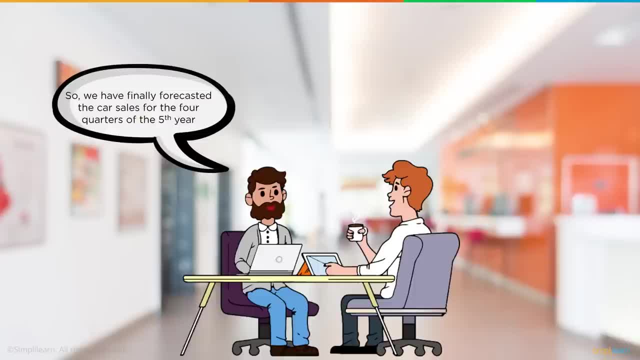 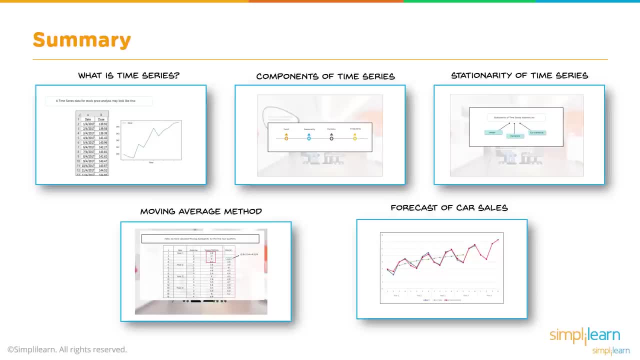 shown versus purely predicted and, as I mentioned earlier, we can safely assume that the values are accurate and predicted properly for the fifth year. now we come to the summary. so what have we seen in this video? we talked about time series data. why time series? what exactly is time series? what are 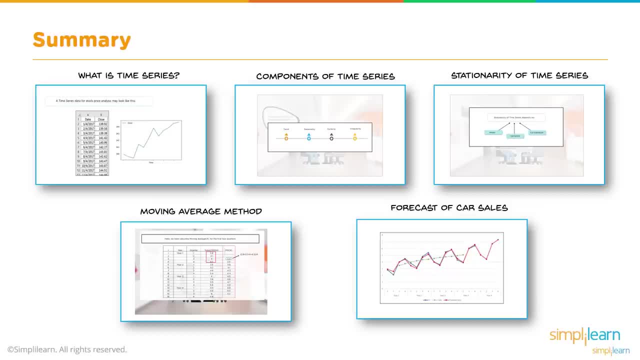 the components of time series data: the trend, seasonality, cyclicity and irregularity, or random. and then we talked about the stationary time series data. what exactly is stationarity? what are the components of stationarity? how do we visualize stationary time series data? and then we use the moving average method to perform.